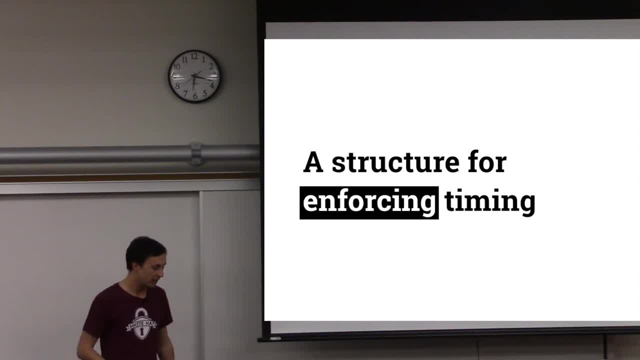 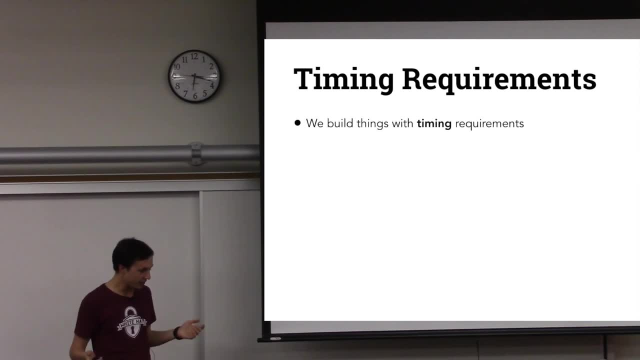 is that it enforces timing between different tasks. you want to do So. we should talk a bit about what kind of timing requirements we want to enforce, And those are obviously. we build things that need to be aware of how much time things take and need to respond. 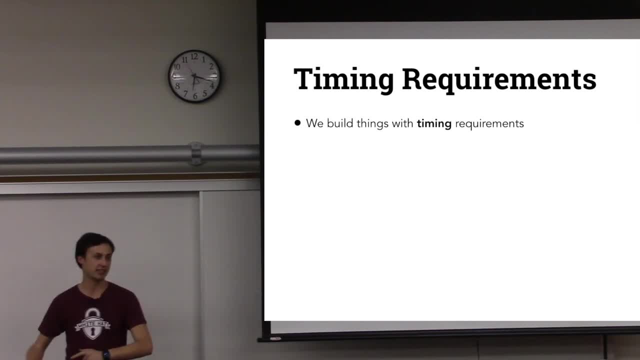 to things in a certain amount of time, need to have events fire off in a certain time frame, But so when we think about timing requirements, we have words to describe them Like are they hard or soft? And basically that means like. 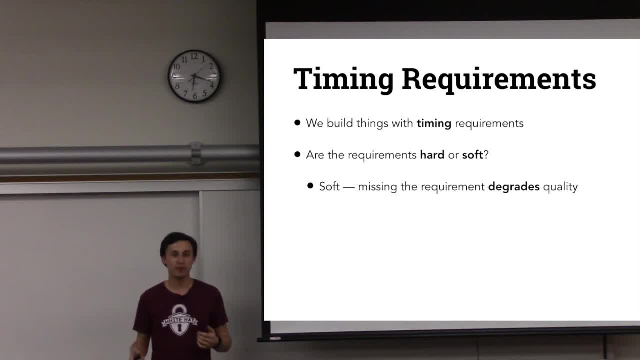 a soft timing requirement means that if you miss the requirement it degrades the quality of the system. So I'm sure anyone that's used a video chat service knows what missing a timing requirement looks like. I mean it freezes, The audio gets choppy, It sucks. 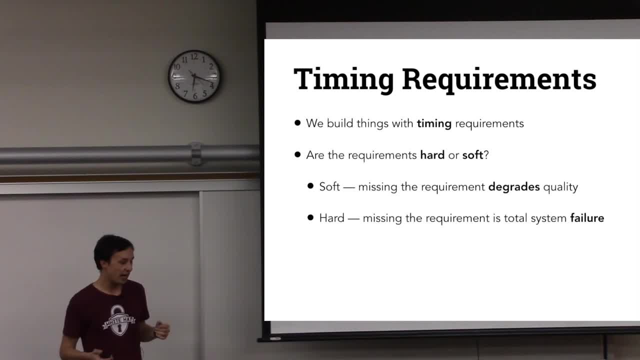 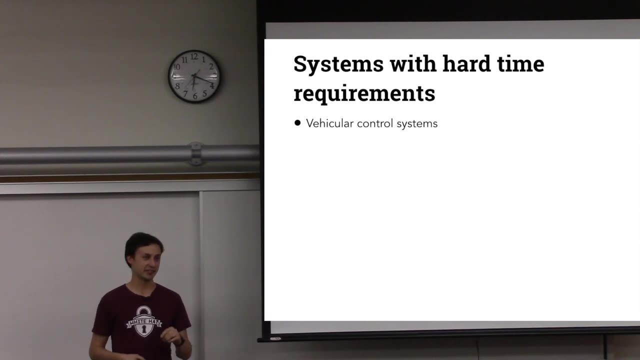 but it still works. You can kind of communicate with it. Hard timing requirements are where missing the requirement results in total system failure. And so what kind of systems have that? Well, obvious ones are vehicular control systems, So like if your car misses a timing requirement, you can crash into the person in front of you. 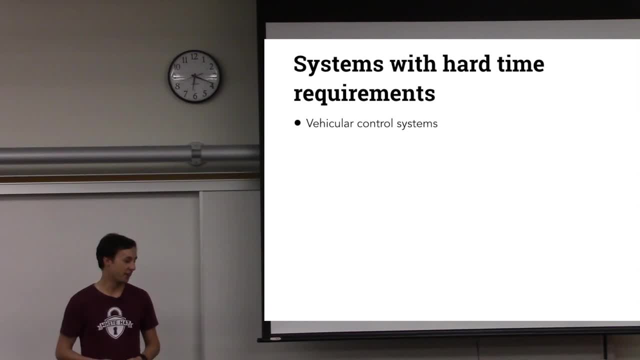 if the brakes don't activate fast enough Or if your rocket misses the timing requirement, then it gets screwed up and goes the wrong way and you're not going to space today. Also, pacemakers and a lot of other medical equipment, obviously. 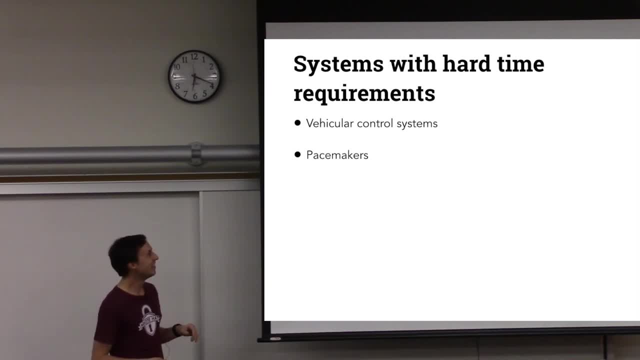 pacemakers have very hard timing requirements, Otherwise you die. Anyone else have hard timing requirements in mind? Jasper? Ah, yes, If you're firing radiation at people, you want to make sure you don't do that too long. 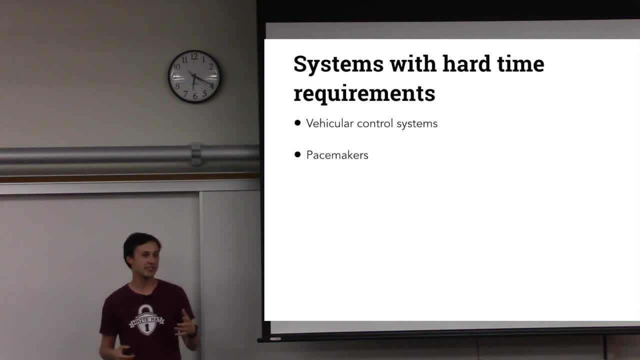 And in general, there's all kinds of systems that deal with signal processing of some sort, And most of the signal processing we do has some kind of isochronous requirement That, if total system failure is a bad thing, you'd want to avoid. Yes, 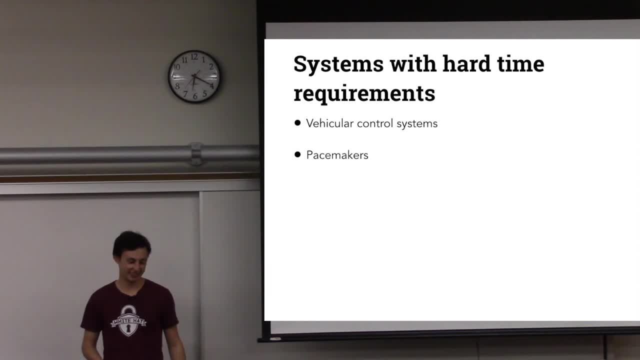 Same time, Isochrone, Yes. So what do we need to do in order to enforce these kinds of requirements? Well, the first thing is measure time, Because, obviously, if we don't know how much time has happened, we can't do anything about it. 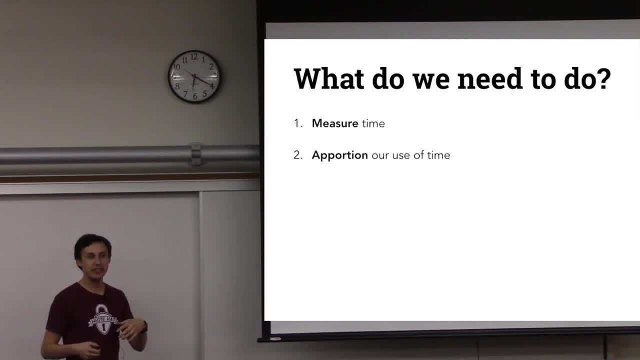 We also then need to apportion our usage of time, So we need to have some system to describe how much time something takes, how much time something should take relative to something else, and how we go about actually deciding what gets to run when on a microprocessor. 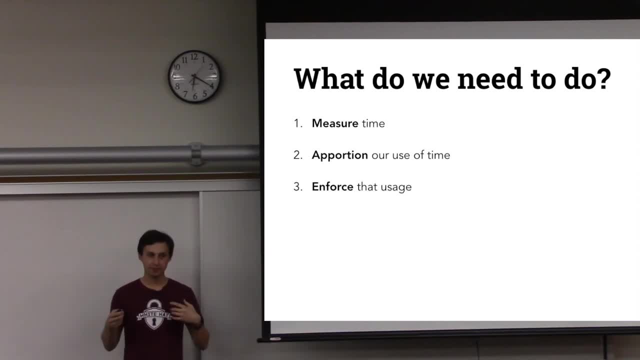 And then we need a system to enforce that usage, to make sure that, if we have described how we want the system to behave, that it continues to behave like that. And finally, we want to make it possible to still do useful things within that structure. 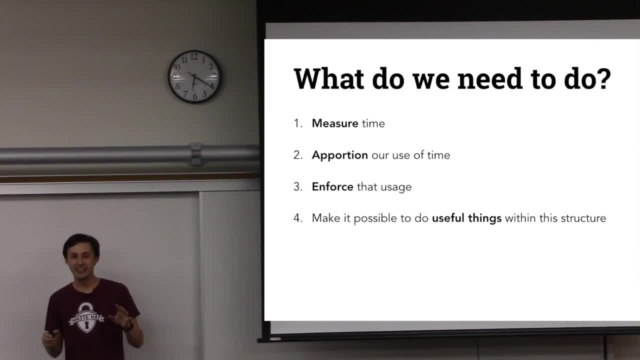 Because obviously, if you measure time really well and then use it perfectly, you might still not be able to build something useful with that. So the first thing we're going to put in the system in order to have time requirements in it is to create ticks and tasks. 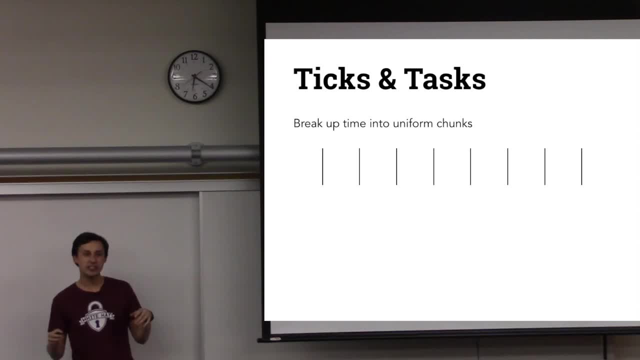 So we're going to break time up into uniform chunks we call ticks, And these chunks are enough time to do some amount of computation in, And that amount of time is flexible depending on how you define the system. All we know is that these ticks will happen at uniform spacing. 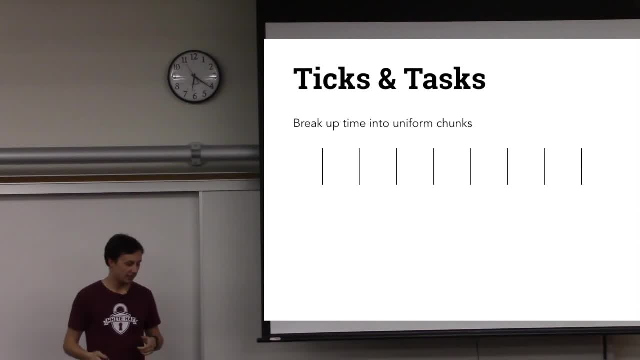 and we're going to be able to schedule a task into that. So we then put our application code into a number of independent tasks So we might have wind the warble, jangler and degauss the T-shirt cannons as two separate tasks. 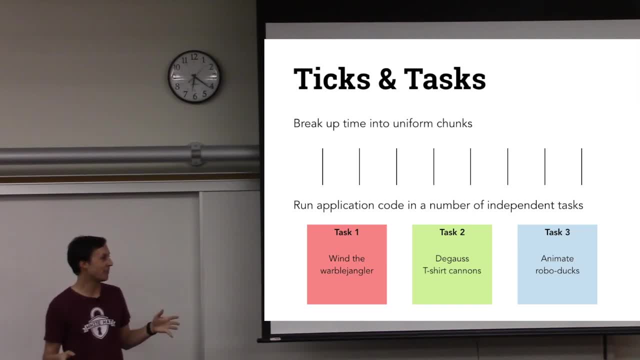 And we want to make sure that the CPU executes both of them in a certain amount of time. Obviously, animating the RoboDuck is animation. We want to make sure that happens regularly. So we have ticks and the operating system is going to keep track of ticks going by. 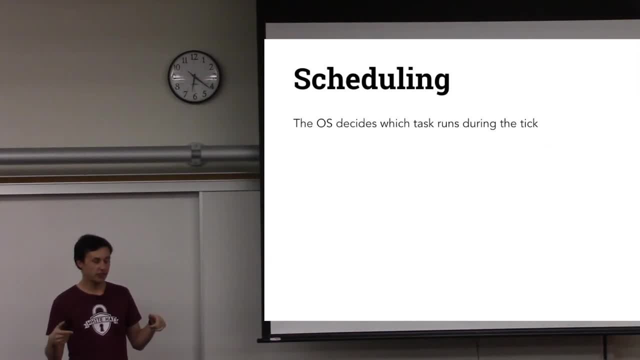 and we have tasks. So we're going to schedule them into the ticks as they go by, And the OS decides which task runs during the tick. So how does it do that? Well, we get our ticks and we have our tasks. 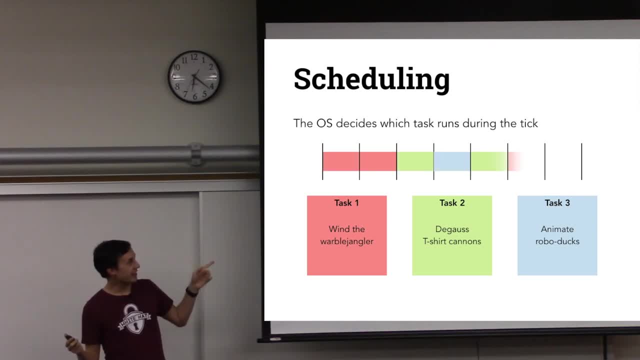 and then the OS is going to figure out: okay, well, it's going to run that task, then that task, then that task, then the other time. And this is pretty common. I mean, anyone familiar with a multiprocessing system knows that the operating system 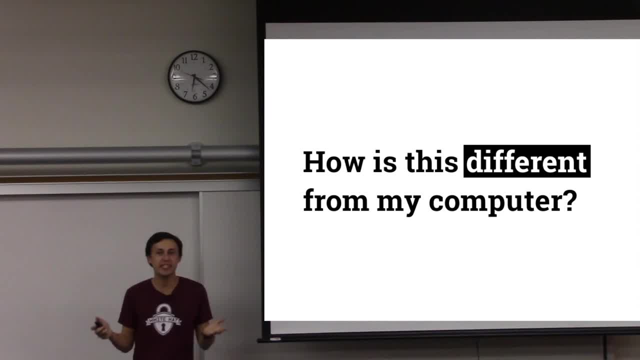 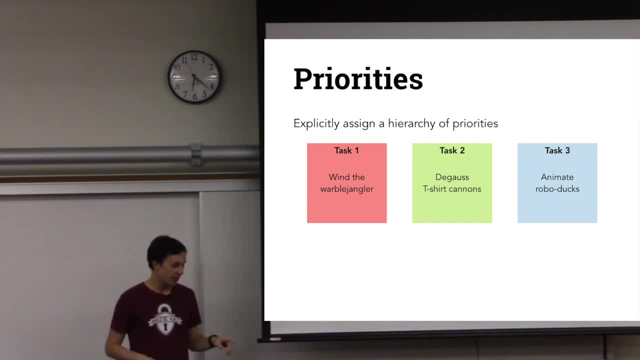 is going to have to swap out processes as we go along. So how is this different from my own computer? And the answer is priorities and determinism. So we explicitly assign to all of our tasks a hierarchical priority ranking And then the OS always runs the highest priority task it can deterministically. 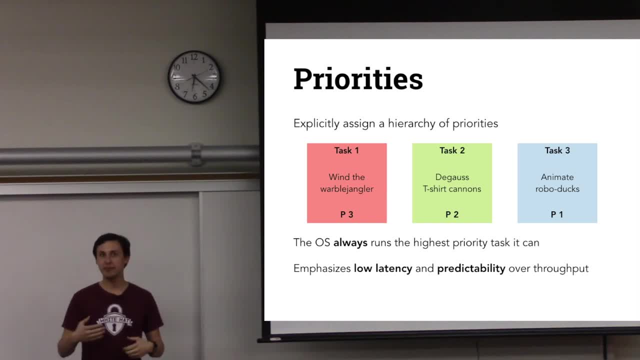 So when we say deterministically, it means that we can predict what the operating system is going to do. And with a hierarchical priority system, it's easy to do that because we can always say: oh well, it's the highest priority task. 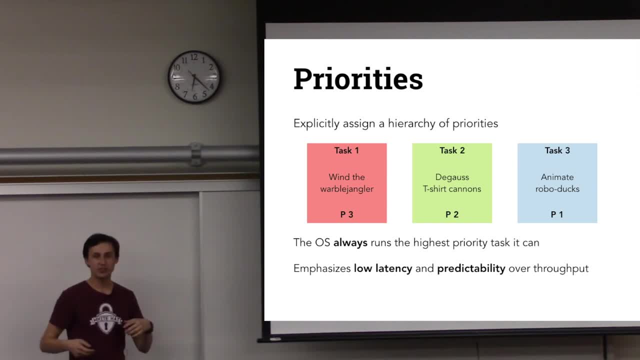 It's always going to be doing that, And this differs from a regular operating system, because, of course, we're抔 system, because, instead of valuing throughput and appearing like it's simultaneous, because obviously a laptop is doing a lot of different things at different time frames, but it's really 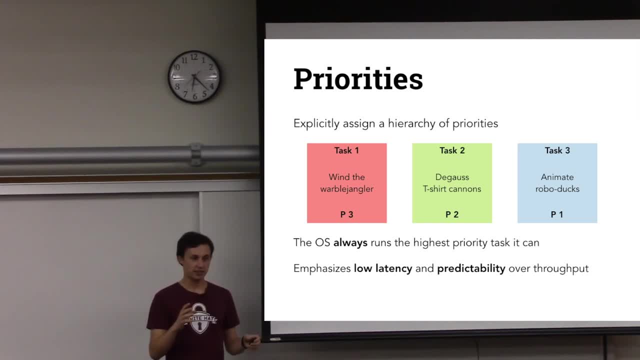 just trying to do as much as possible without sacrificing too much of any other task. In an RTOS. we want to have low latency and predictability, So we don't want the operating system to suddenly say: oh well, priority two hasn't run in a long time. I should make sure. 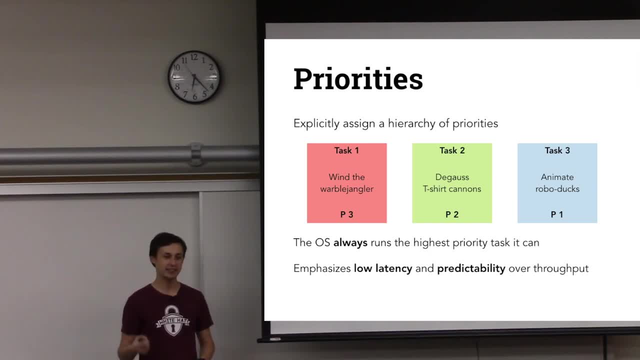 that actually gets updated. No, as long as there's a priority one task, the system's going to run that task. So when we create our ticks, in this case all these tasks are running, but the priority one task is there. So when the system runs these tasks, it just runs all the blue tasks. 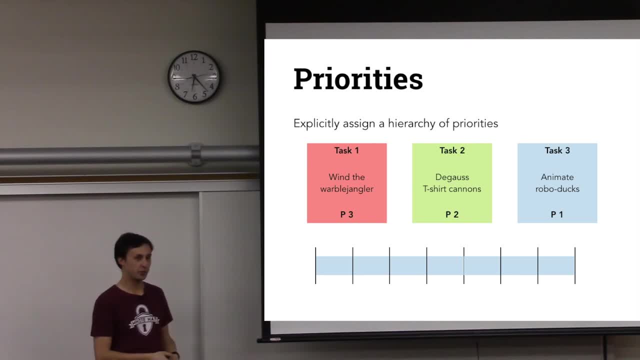 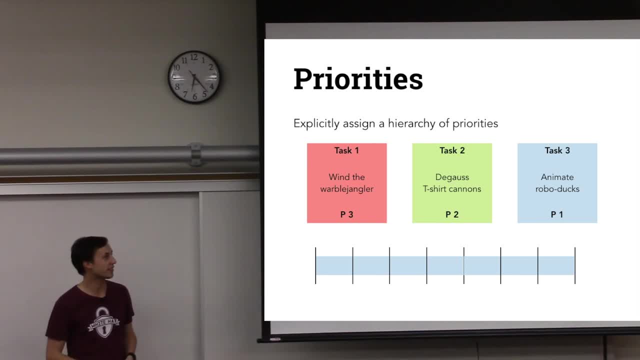 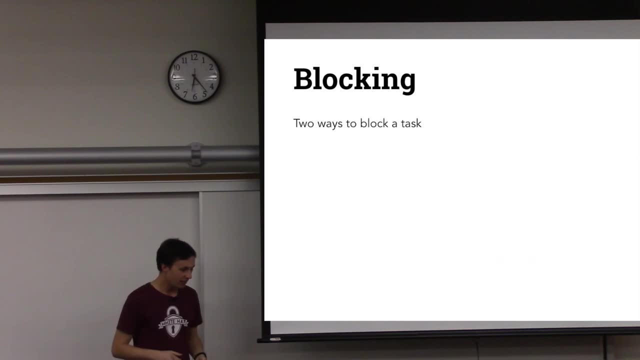 How do we stop this from happening? Because obviously we don't want to neglect our warble janglers or t-shirt cannons, So for that we introduce blocking. So there are two ways at least. I'm going to be talking about free RTOS in this talk, because it's a relatively 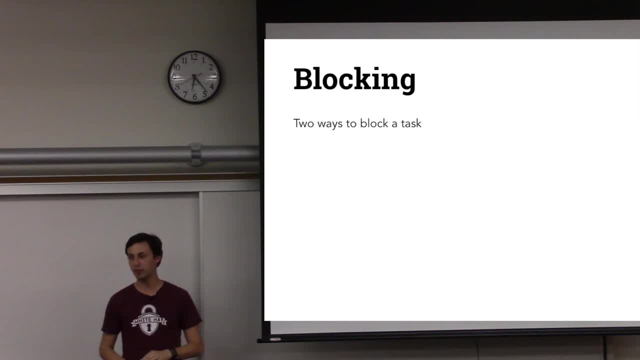 minimal free, open source implementation of a real-time operating system. You can just go use it. So everything I talk about in terms of exactly what constructs we use is taken strictly from free RTOS, And that's completely not because that's the only operating system I have experience. 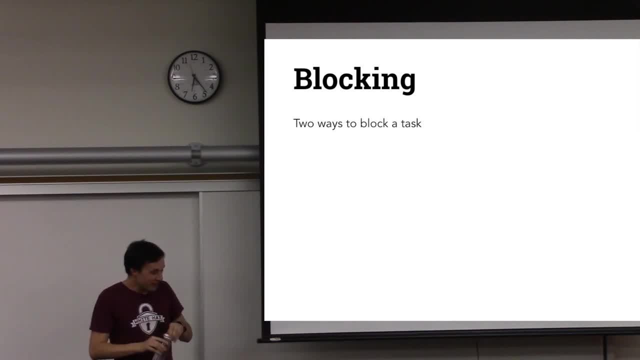 in. So we have two ways to block a task. One is explicit delays. So that's where we have in our task a hook into the operating system to say, hey, don't run me for another number of milliseconds. And the other way is intertask communication. So if we want to talk to another task, 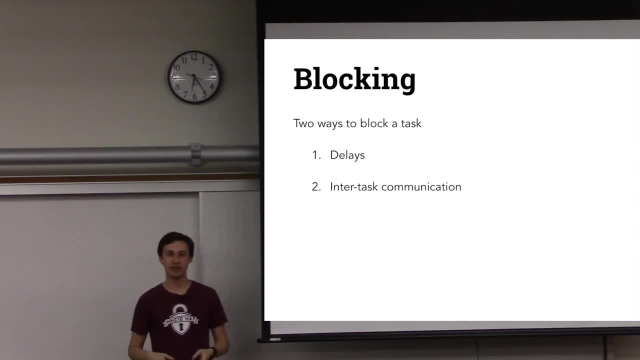 we can block on receiving information from that other task. So as long as we're waiting for some piece of information from another task, we can choose to just sit there and wait until it's handed to us. So our previous rule was: the operating system always runs the highest priority task. 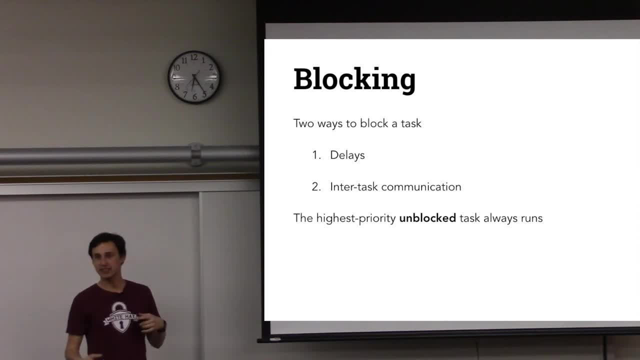 It's actually it runs the highest priority unblocked task, And so that's how we get lower priority tasks to run. We always handle the highest priority tasks until they block and then we go down. So let's talk about an example of some kind of system we'd want to build. 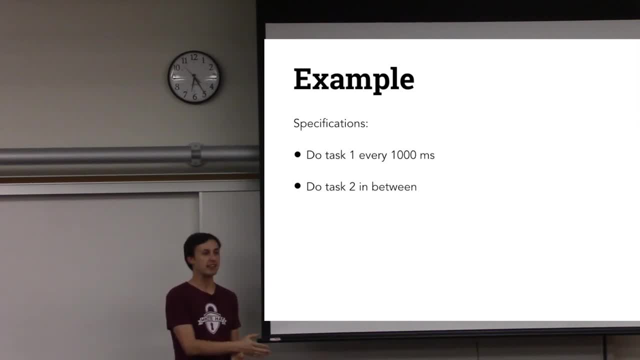 We're going to have two tasks. One we want to run exactly every 1,000 milliseconds, or at least as close to that as possible. We can figure out a way to build our system so that it only happens plus or minus a certain number of milliseconds, but it always happens. 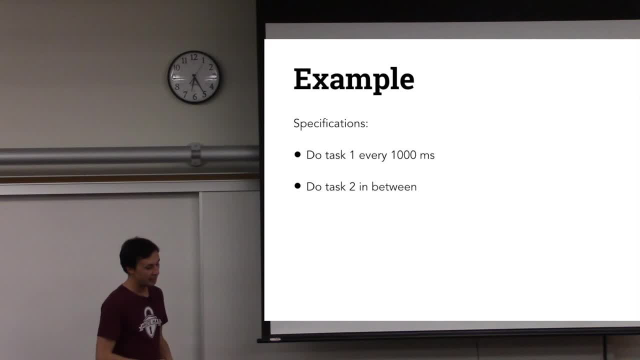 almost exactly 1,000 milliseconds apart, And the entire rest of the time we just want to be running task two. So maybe the t-shirt cannons need to be degaussed every millisecond, but the animation. we can get the highest frame rate if we just run in between that. 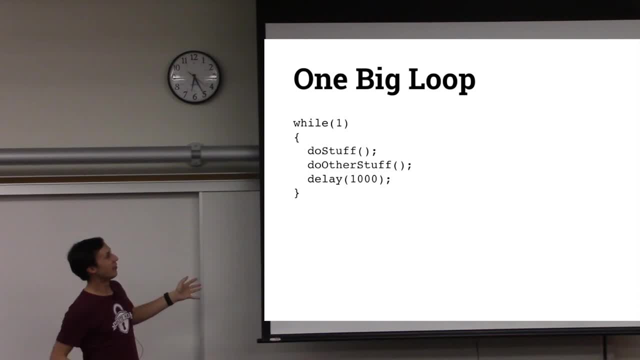 So the first thing we might do, The first thing we might do is just get one big loop where we do stuff and we do other stuff and then we wait a second And this works. but when we have task one and task two and then a, 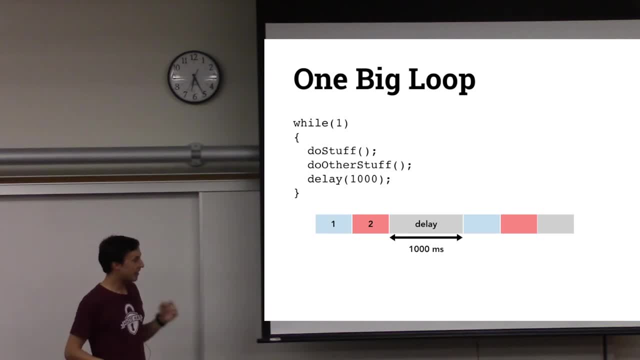 delay. the delay is 1,000 milliseconds, yeah, but task two takes a certain amount of time and it would suck if we had to hard code that into the delay. We don't want to be like: oh yeah, task two, we measured it. Task two takes this amount of time, so we'll just subtract that. 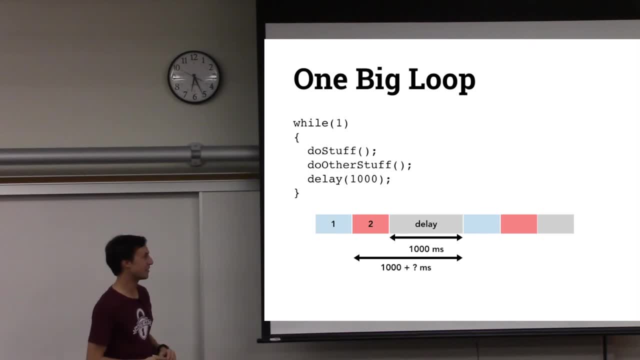 from 1,000 and keep going. That's bad. So the other problem is task two might not take the same amount of time every time we run it, So it might not even be possible to hard code the amount of spacing we want in. 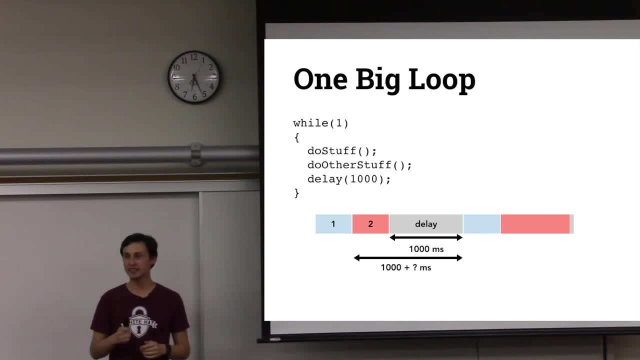 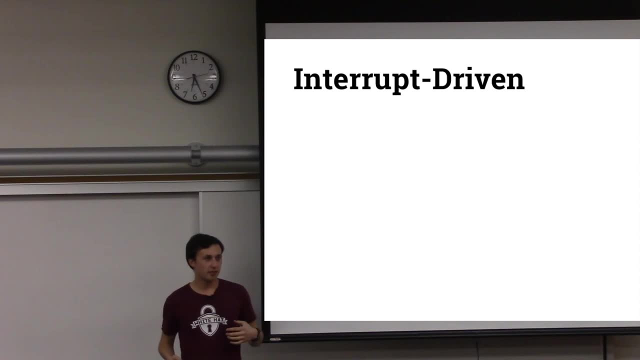 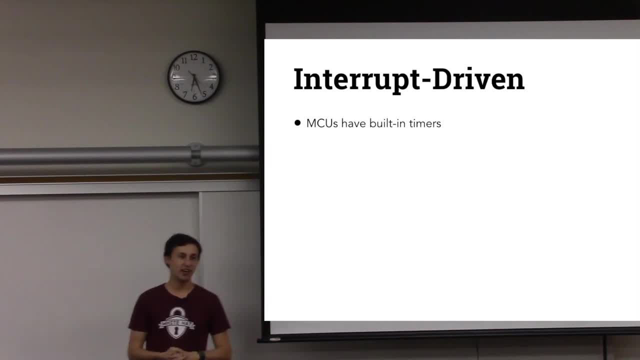 go over that Microcontroller. So microcontrollers have a bunch of hardware built into them And because they're really small embedded systems, we can often just reach directly into that hardware and say: do this. And so MCUs often have a number of timers in there which will trigger an. 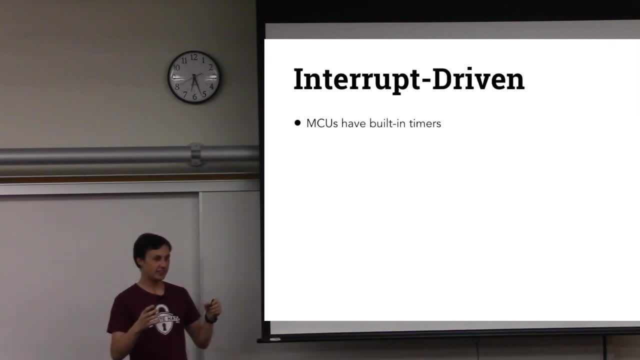 interrupt, And so the interrupt means the CPU stops whatever it was doing at that moment and goes and runs this specific function that we defined at compile time, which is stored at a specific spot in memory, And so we can configure a hardware timer to have the exact delay we want. 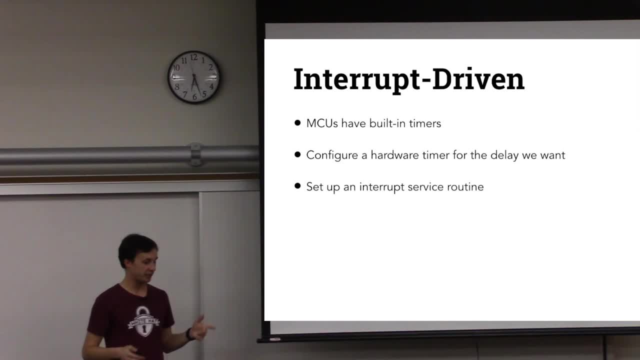 in between tasks And then we can set up an interrupt service routine to actually run the T-shirt cannon degauss every one second exactly, And so that might look a bit like this: where we have our main function, It sets up the timer, And that's going to be a lot of. 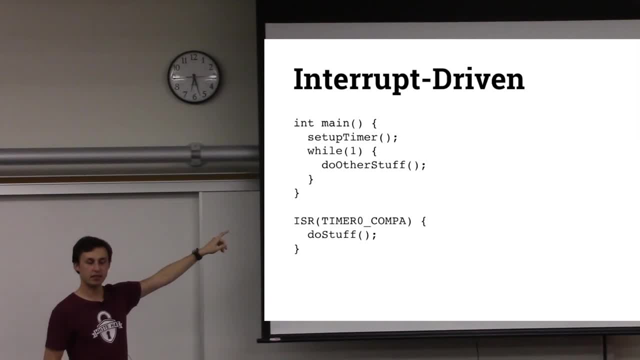 bit twiddling and stuff. Yeah, We're not doing an RTOS solution yet. We're working up to why an RTOS solves this problem really nice. So in this case, the system always treats the interrupt as the highest priority task. So in this case, we set up our timer and the 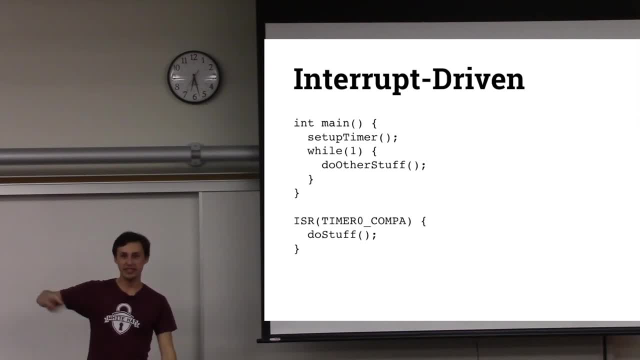 interrupts and everything so that it actually works, And then we just run the task two while we wait for the interrupt to happen. And as soon as that interrupt happens, we degauss the T-shirt, cannons and then go back to doing the other stuff wherever we left off. And this works really well. 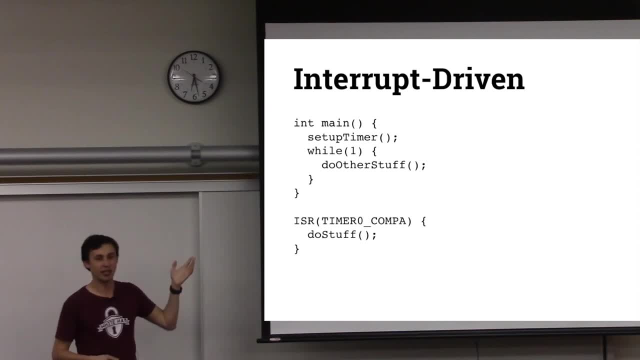 In fact, most of the time, we don't have to do that, We don't have to do that, We don't have to do that. If you're dealing with an embedded system, you have a lot of interrupts going on in it, In fact. 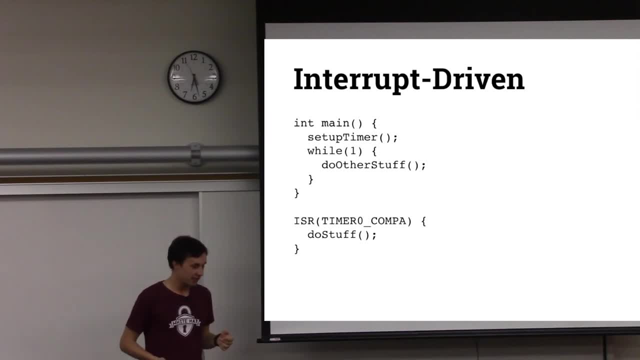 RTOSes use interrupts all the time, But the problem with this is like if you want to have a lot of tasks and you want to run this code on a lot of systems, this particular solution isn't portable. Each microcontroller is going to have different interrupt handling, different timers and might. 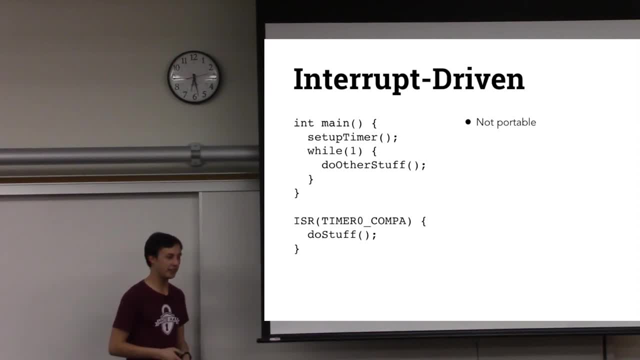 even be running at a different clock frequency, And so it would be really nice if we could figure out a way to describe these tasks and figure out how to have it. It would be really nice if we could get the RTOS to do it. But it would be really nice if we could get the RTOS to do it. 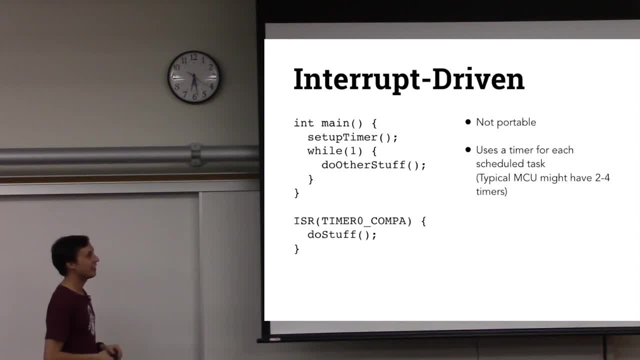 The other problem is if we want an interrupt for every task, the hardware usually only has so many interrupts, And so if we can utilize just one interrupt to schedule tasks and leave it at that, we can have a lot more tasks running on the same microcontroller. This is also pretty hard to. 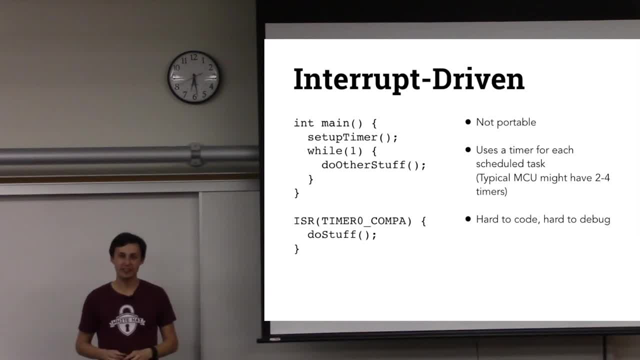 code. I don't think anyone that's ever written interrupt-driven code has been like, yeah, this is the easiest thing ever, It's absolutely necessary. Don't get me wrong. But it's just sucks to have that mental overhead when you're trying to design a system to do a thing. 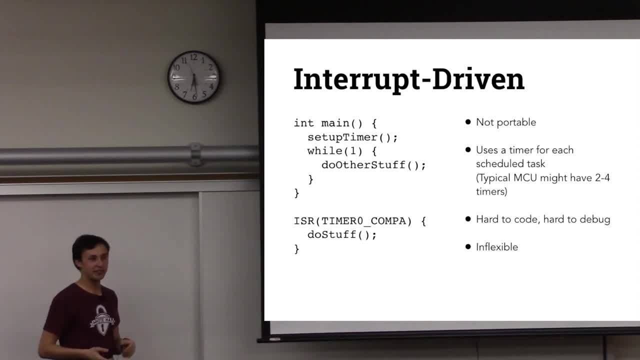 nicely. It's also really inflexible. If you want to add tasks and rearrange them, you have to completely restructure how your timers and interrupts work. And lastly, like I said, the RTOS has already invented this wheel, So let's talk about how 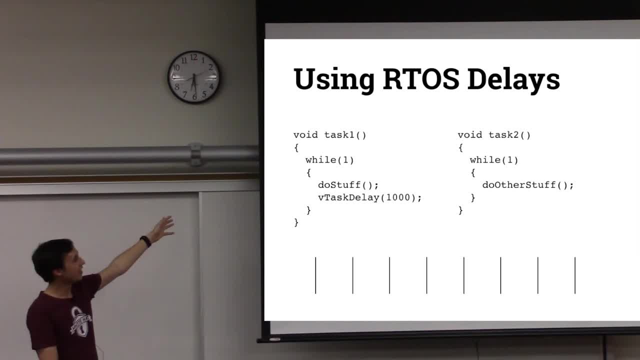 we do this in an RTOS. We have two functions. Task one does stuff and then calls into the operating system with VTASK delay and waits 1,000 milliseconds. Task two: just does stuff, does other stuff, And so when the operating system schedules this, we get task one running. 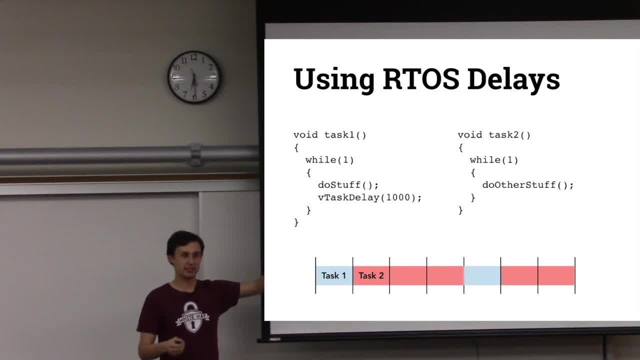 and then, roughly a thousand milliseconds later, modulus the tick length, you get task one running again. So we have multiple tasks, Task two running while task one is blocked, because when we create these tasks in the operating system we say hey, by the way. 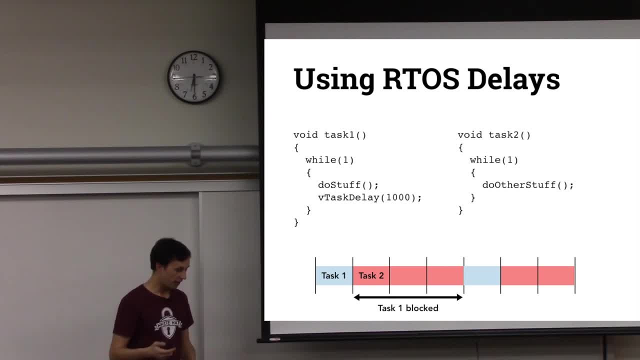 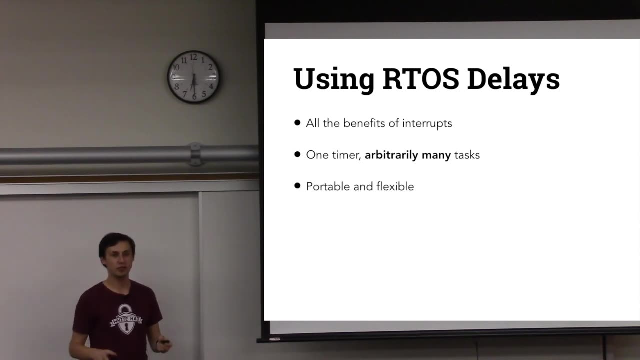 task one is priority one. task two is priority two. So RTOS delays give us all the benefits of the interrupt-driven design. Using exactly one timer, we can schedule arbitrarily many tasks And it's portable and flexible. As long as you've written the code for the operating system, you can move it between microcontrollers. 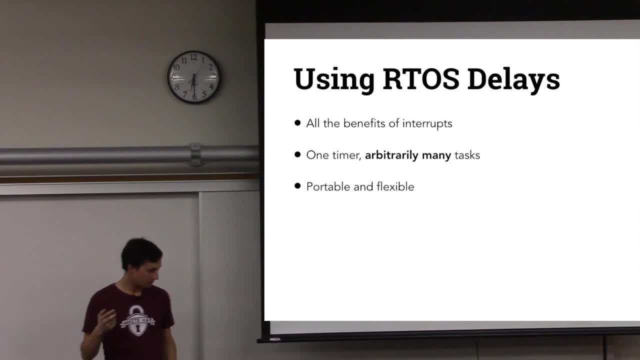 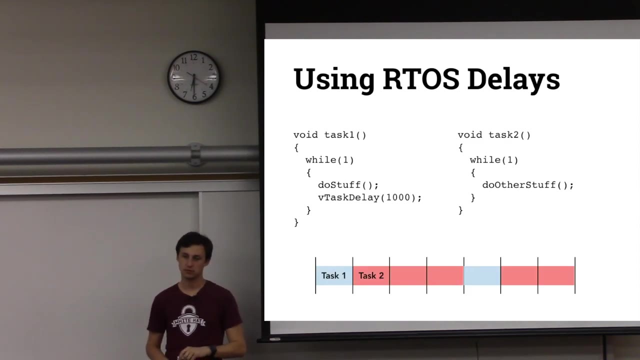 and it will run the same way on each. So the other kind of yes, So could you go back a little Mm-hmm, So that kind of fits At the tick boundary. Most RTOSs use a preemptive scheduler, So we set up a timer. 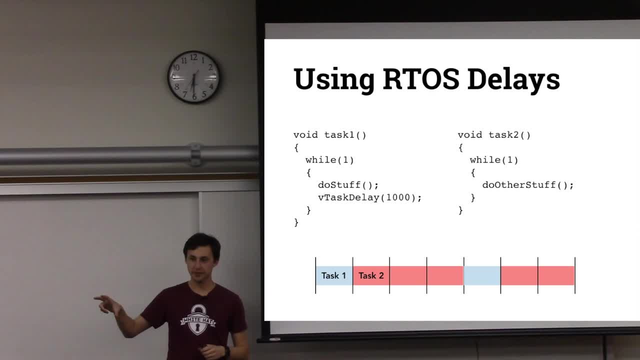 on the microcontroller to call in to trigger an interrupt And then that interrupt calls the whatever scheduler process is in the RTOS And that scheduler swaps out whatever code was running. So I guess in this case it would be just sort of queuing in at the beginning of that. 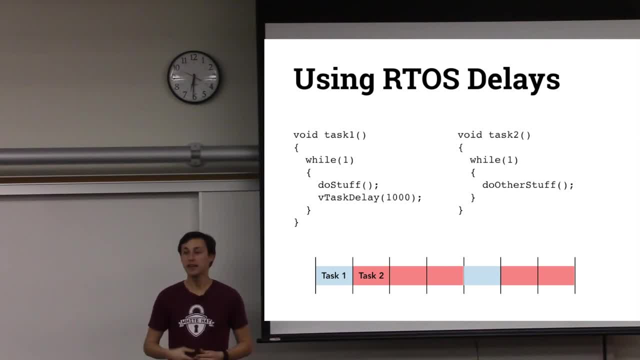 task two. Yeah, In fact, if you look at RTOS timing diagrams you can see task one and task two are running in between, But then the interrupt fires and there's an operating system task that runs. So the system task runs at every tick. 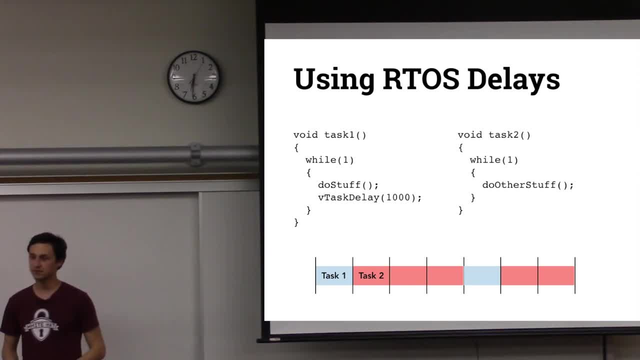 Yes, OK, Cool, So you have ticks inside of task two. OK, Yes, Yes, In between, At this line you can see it's running at every tick. OK, So you have ticks inside of task two. Yes, 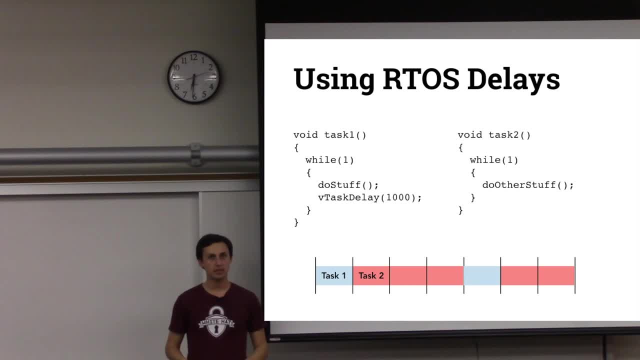 OK, OK, OK, OK, OK, OK. So once this line, task two, is interrupted, the operating system decides whether task two should still be running. And then, when the operating system decides that, yes, I have nothing better to do, task two keeps running. So all the best fits arbitrarily. 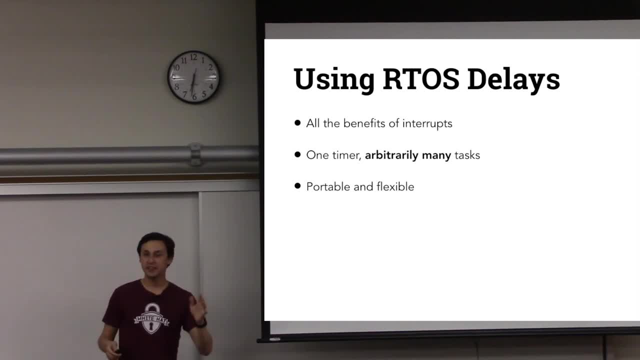 many, and it's portable and flexible. So the other kind of blocking we can do in FreeRTOS is intertask communication And there are two different methods in general for this in FreeRTOS. One is semaphores, where you literally just say: it's just a binary flag, So you just hand it to the task you want to. 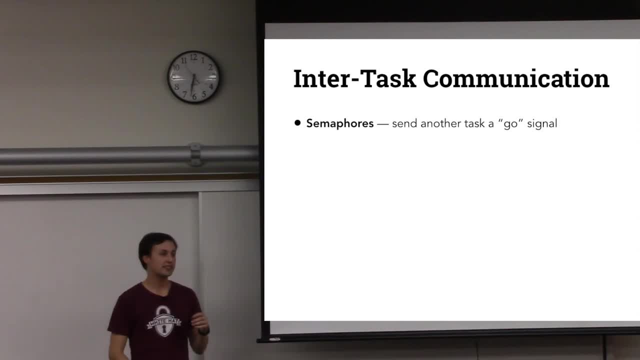 run and it says go, So a priority one task can wait on a semaphore from a lower priority task and be blocked on that semaphore while the lower priority tasks are done and then hand it back So you might have a low priority task that says well, what's the next highest? 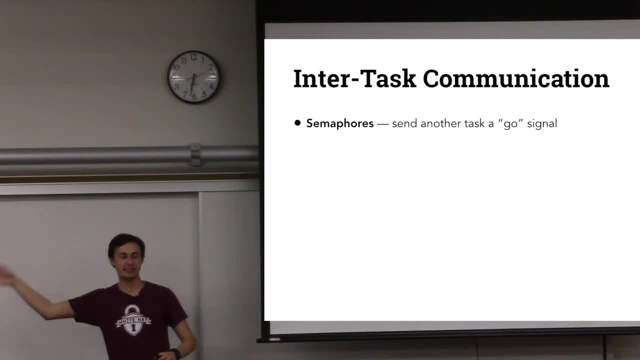 priority And then it rearranges the priorities and hands off semaphores of the tasks that need to run. Would you maybe upgrade the priority of the task that a higher priority task is blocking on? Yes, In fact, when you're designing a system with RTOS, there's a problem called. 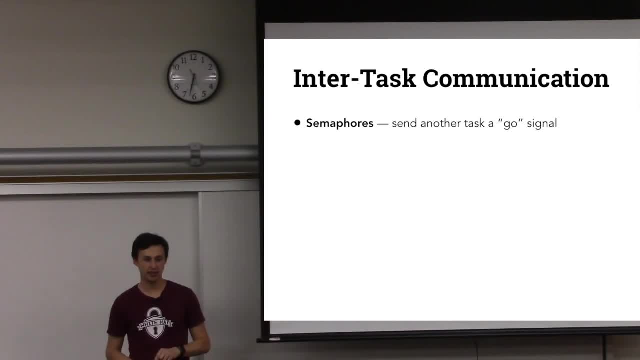 priority inversion, where two tasks are. actually you only need three tasks. I had an interview question about this and I didn't get it right then either. Basically, if you have a shared resource, that a low priority task gets a mutex on, then the higher priority task blocks on. 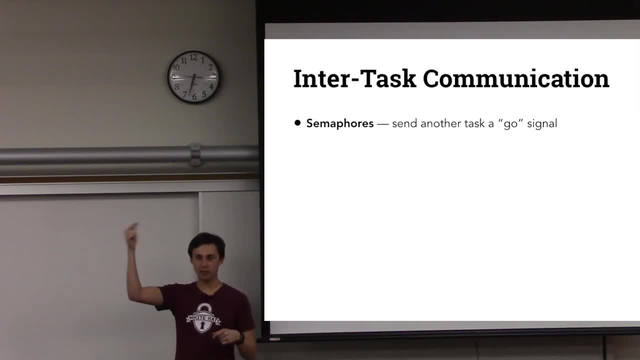 that mutex and you get priority inversion, where the higher priority task is blocked but the lower priority task is running anyway because it has the mutex. The other kind of communication we want to talk about is queues. So queues are basically a first in, first out way to send data to another task. So you can just say: here's a thing. 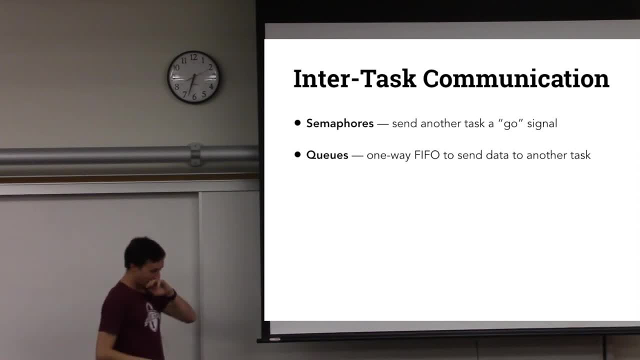 Here's another thing. Here's another thing. Keep working on that, And so both of these works facilitate blocking and scheduling. So any time you want to make sure that you communicate to another task and you don't want to run that task until you actually have. 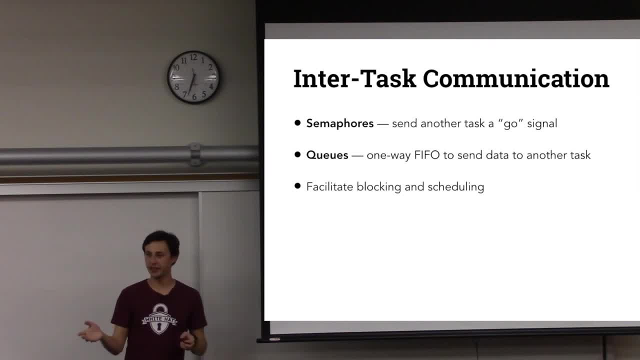 data from another task. you can block on that input and wait for the communication to happen before the next task gets scheduled in. So, yeah, we'll block and wait on the go signal, or block and wait on more data to come down the pipe. 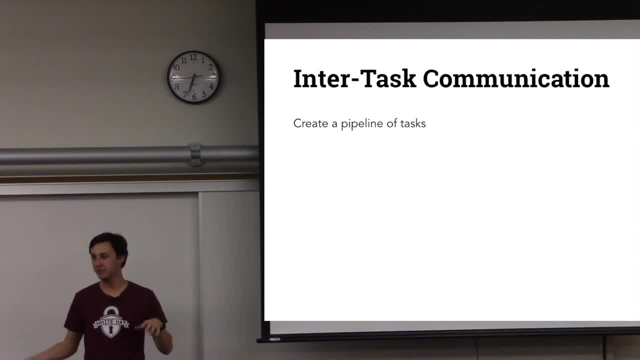 So let's do an example of what kind of communication pipeline we might build with these things. So we have three tasks. One receives a packet from whatever physical device the microcontroller is attached to. The next processes that packet And the receive packet task hands the packet. 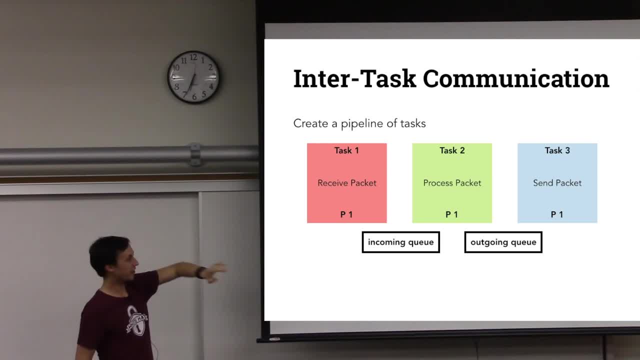 to the processing task in the incoming queue And then we have a third task that gets handed the packet through the outgoing queue and puts it back on whatever physical device is doing the processing. So the pipeline looks like this: So we get the arrow and it's going to the queue and the packet, and the queue and the. 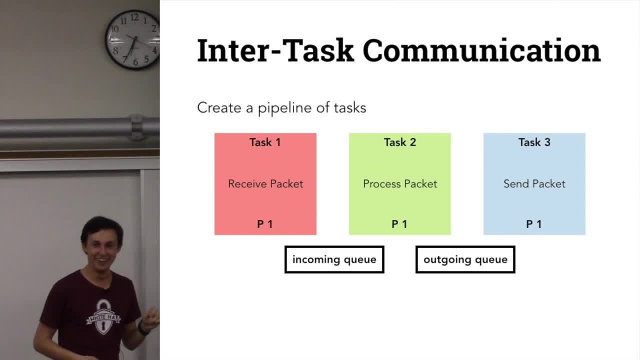 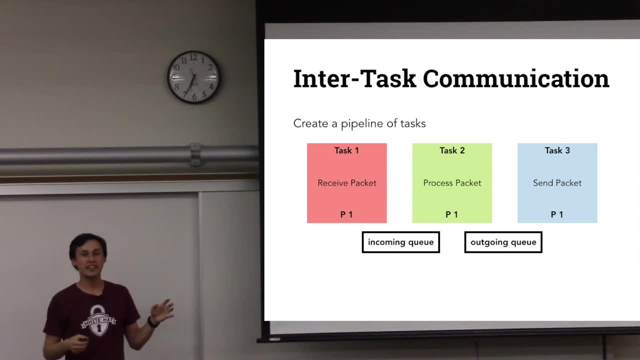 packet and I spent like 20 minutes on that animation, Thank you. So the real cool thing here is each task only has to worry about its own thing And at idle the system doesn't have to care about processing or sending the packets. So the receiving packet 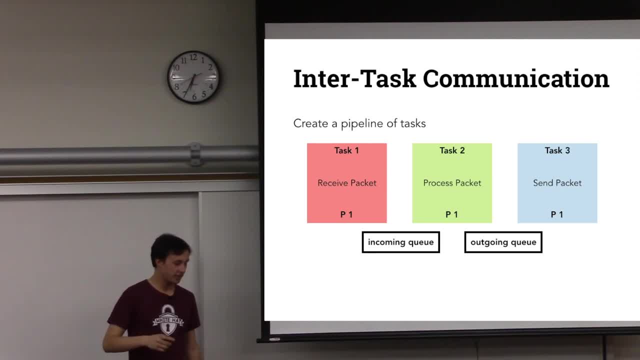 isn't blocked on anything. It can just keep pulling the device And the other two tasks are just blocked. Wait for the packet to come down And then we have the other two tasks. They're waiting for the queues to become full, So at idle you get to see the arrow again. Good, I spent time on it. 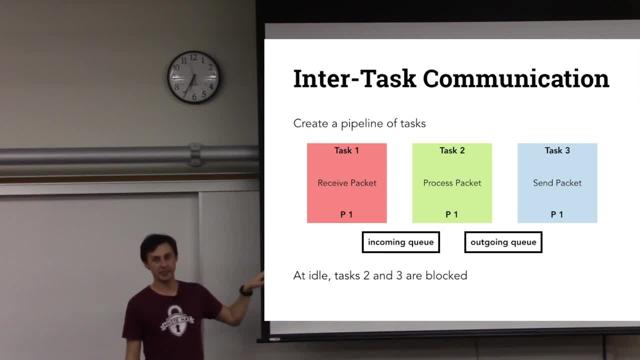 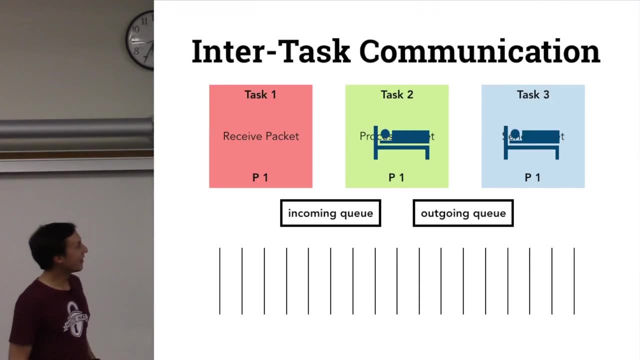 So at idle, tasks two and three are blocked on waiting for input on their queues. So what does this system look like in the scheduler? So at idle, tasks two and three are blocked because task one hasn't received any packets. So we get a packet. 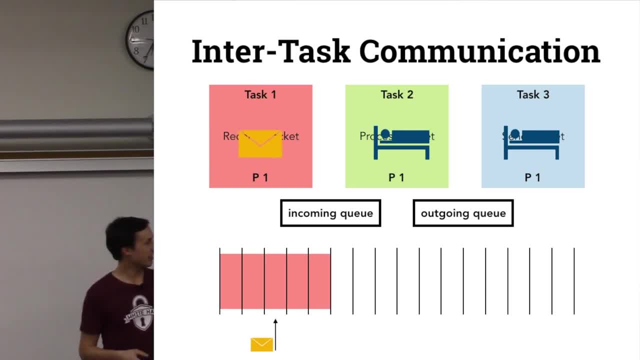 And task one pulls it off the PHY And so during ‑‑ it's at idle for these two ticks. It receives the packet during the third tick And then the next two ticks, it processes the packet and puts it on the queue. For the sake of argument, we'll say that each of these 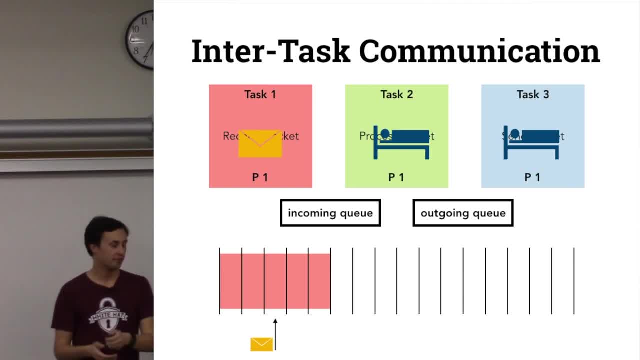 tasks is able to actually do its job in two ticks. So once task one processes the packet off the PHY and puts it on the queue, it hands it the queue and task two wakes up. So during that time ‑‑ Task one and two are both unblocked. 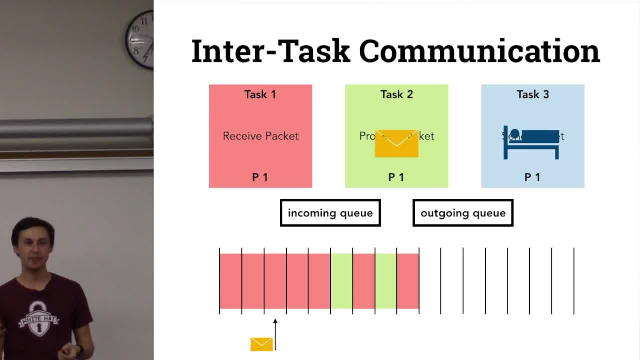 Task one waiting for another packet to come in. So even though we're processing the packet, we can still be pulling one off the PHY. Task two is processing the packet, so they trade off time slots. The exact way it trades off is a matter of how you design your scheduler or what kind. 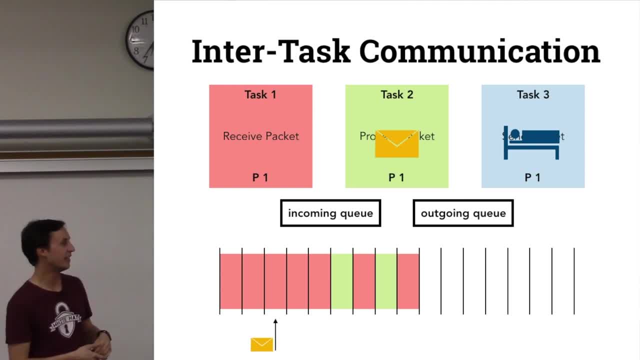 of options you choose for your scheduler. So if you design an RTOS system, you can make all kinds of choices about how you want scheduling to happen. In this case we're saying they just trade off time for whatever tasks are currently unblocked. 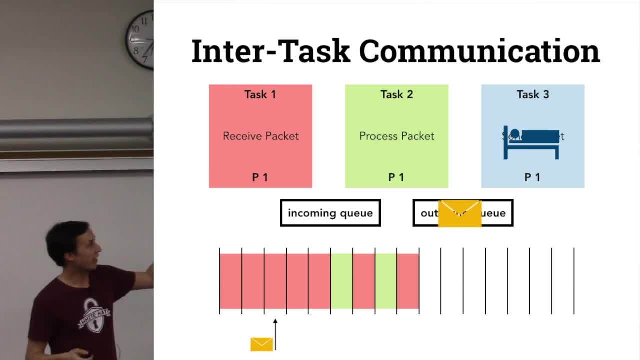 Task two processes the packet and puts it back on the outgoing queue, at which point task two goes to sleep because its queue is empty, But task three wakes up. So task three and task one trade off time, while task three sends the packet back out. 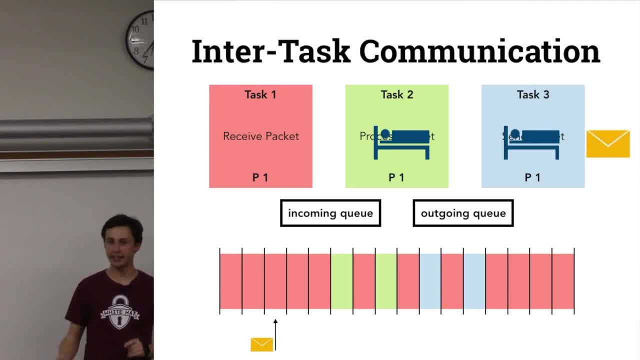 onto the PHY, And then we're just left with task two and three at idle Task one waiting for a packet to come in, And so this is what happens with a single packet passing through. But obviously the whole point is that we can scale up to tons of packets flying at the 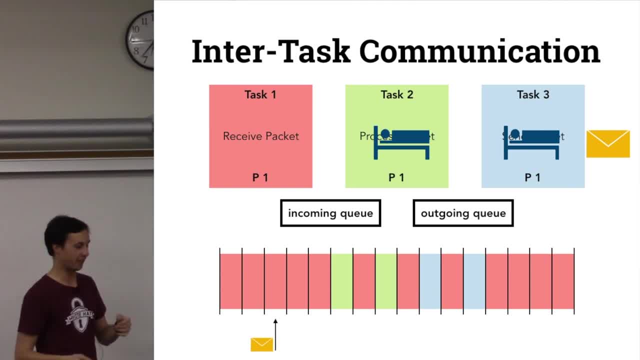 system all the time And to some degree processing all of them at the same time. So if task one has a bunch of packets on the PHY- whatever physical buffer is built into the device- and task two has a bunch of packets on its queue, then they can share time processing. 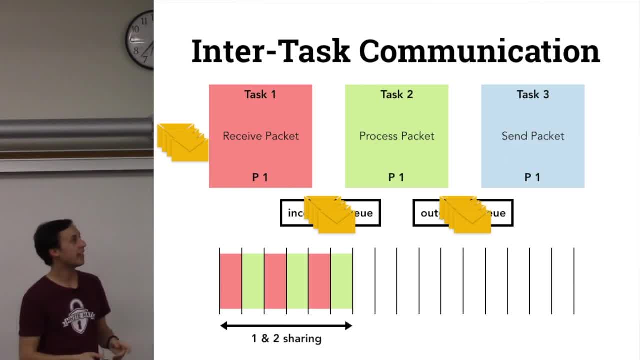 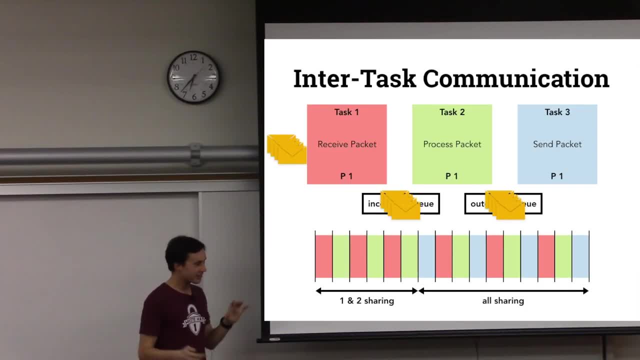 packets. And as soon as task two puts packets on the outgoing queue, task three wakes up and they all timeshare for the rest of the time, clearing their buffers in turn. So this is all great, But what's the point? Why is this special? 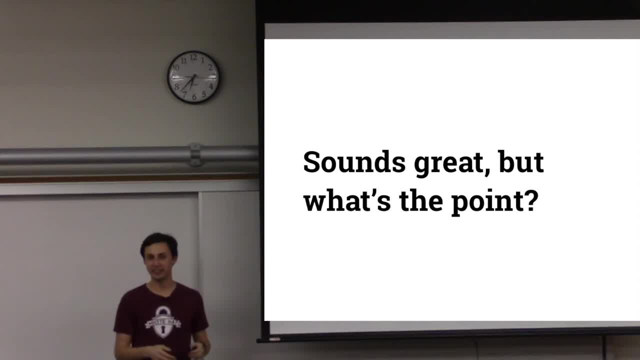 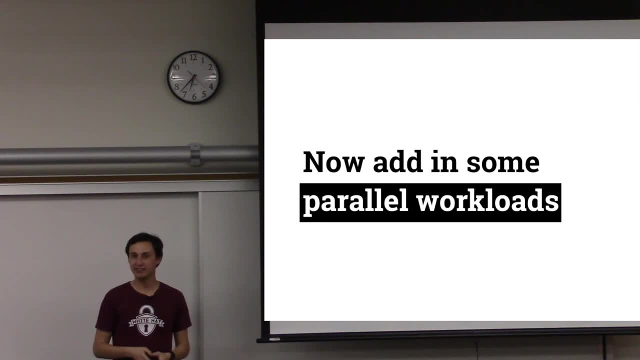 Like we can easily design a system that does this without an RTOS eating up time in between these tasks. Well, what we're going to do now is add some parallel workloads. We want to do all that simultaneously with some other thing. 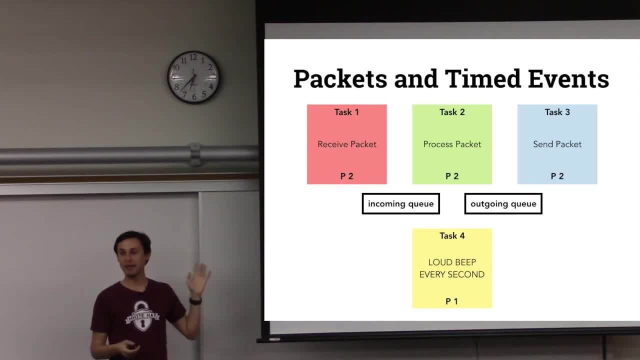 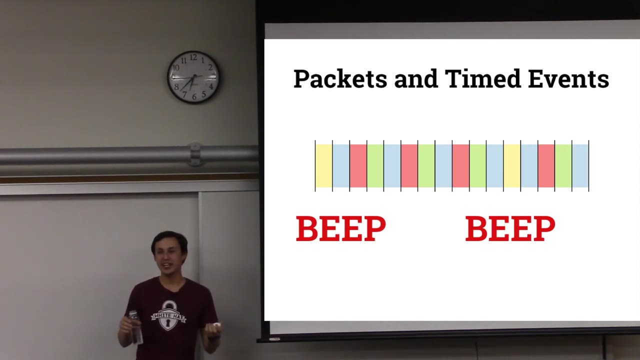 So we'll have our packets and we'll have a timed event where we want it to beep really loud every second. It's really important that it happens every second. So here's our ticks and here's the scheduler. All right, And so this is really great because we can design our packet processing system so that 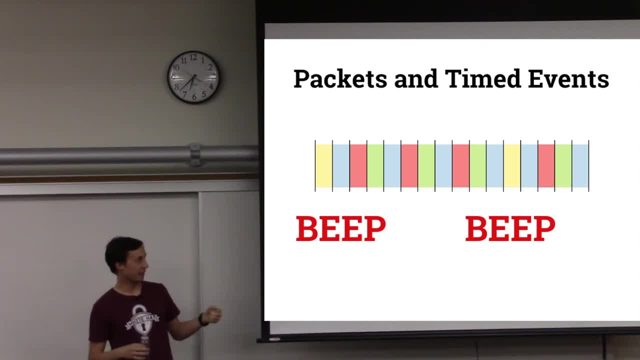 it meets all its timing requirements And all we have to do is know that one tick every once in a long while is going to eat up. one is going to be eaten up by the beep task. We don't have to worry about how the beep task is going to interfere with the processing. 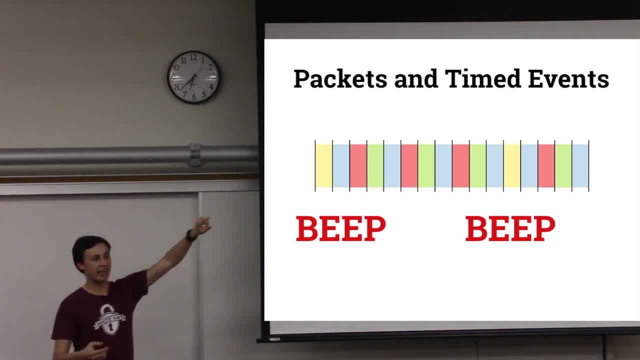 pipeline. We don't have to be like, okay, well, we check the PHY, we process the packet, we send it back out, we check whether we need to beep and then we do that again. We don't have to worry about how that's going to work. 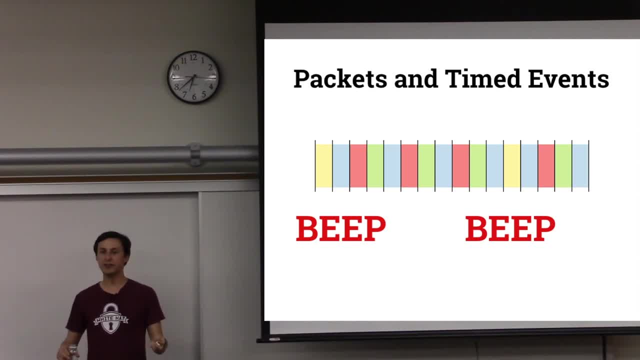 It's going to affect the timing of those things. We know that the beep is going to happen every second, regardless of how long it takes to process a packet or put it on the PHY or what have you. And the other thing is, since we don't spend any time checking whether we need to beep, 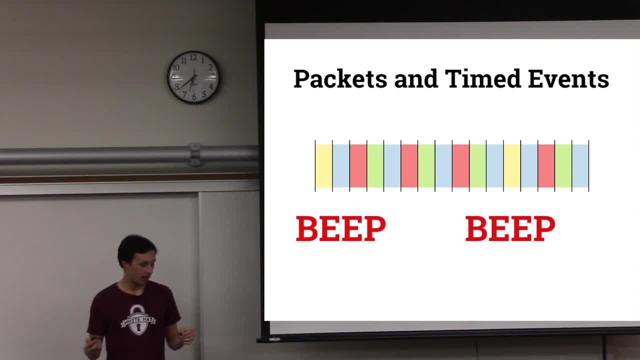 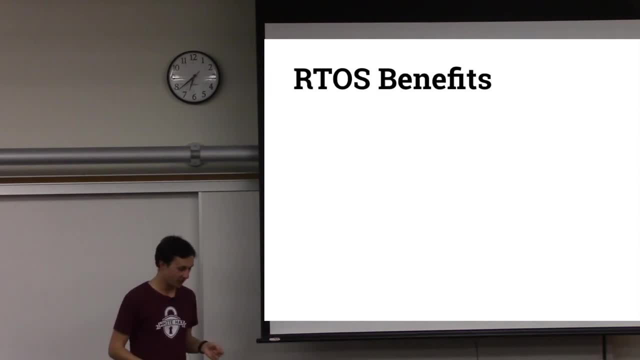 except for whether the process is unblocked, we can use all the time in between to process packets. So there's a lot of benefits to using an RTOS. It makes it really easy to process parallel workloads- Okay, And also to have each workload dynamically scale back when idle. 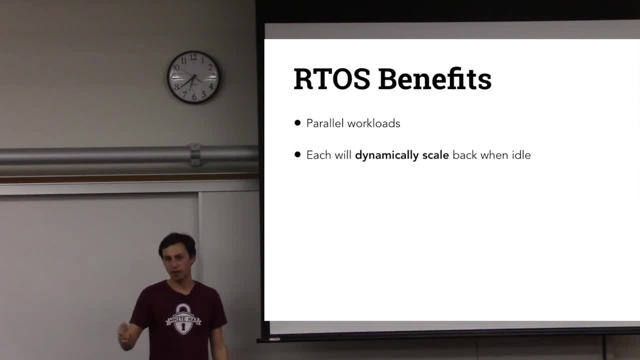 So when we don't have any packets coming in, the system, idle task will run and we don't have to do anything. We can just focus on: do we need to beep, do we need to beep, do we need to beep? Or if we have multiple different processing pipelines going on and one's really busy. but 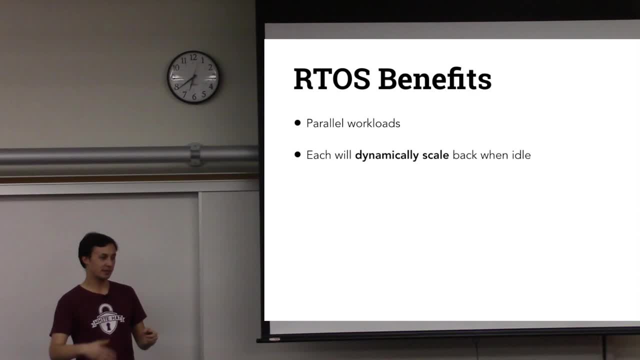 the other one doesn't have any activity, we're not even worrying about that. The system is putting all its work on the workload that has a lot of work to do. The other thing is Okay, So we can have low priorities for the system automatically preempted by high priority tasks. 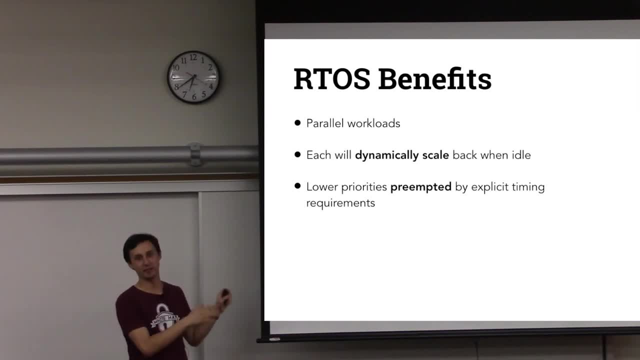 based on explicit retirement requirements which we set up when we program the thing. So the system will automatically shift its workload as it needs And it isolates the processing of independent subsystems. So we can have multiple things going on and we don't have to worry about whether my processing 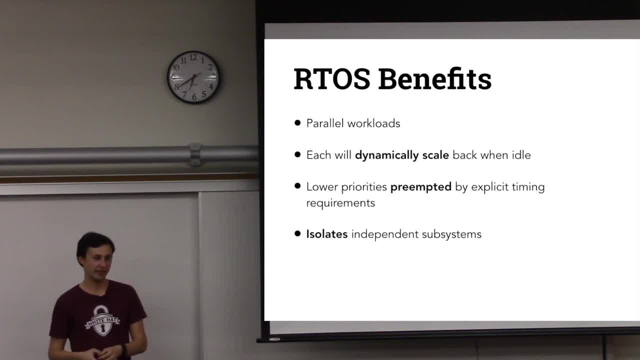 here will affect that other thing, unless we get super time constrained and then we have to be like, well, okay That one can't run now. So it's really good for making sure that we don't have overlapping design requirements in our head at any given moment. 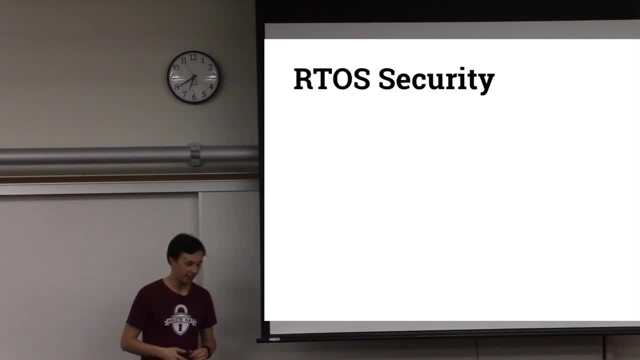 So let's talk about what RTOSs do for us in terms of security, And the answer is not really much other than that they're really useful for helping you think about what you need to do next instead of how you're going to make the timing requirements. 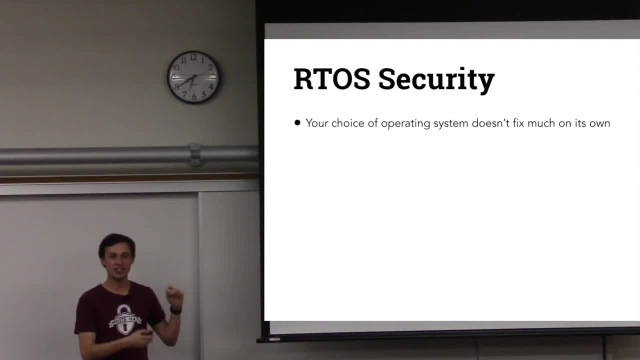 work. That's because The choice of operating system, at least in terms of RTOS, doesn't really fix all that much on its own for all the things you have to worry about in an embedded system, Because the RTOS doesn't fix your boot ROM integrity or firmware updates. 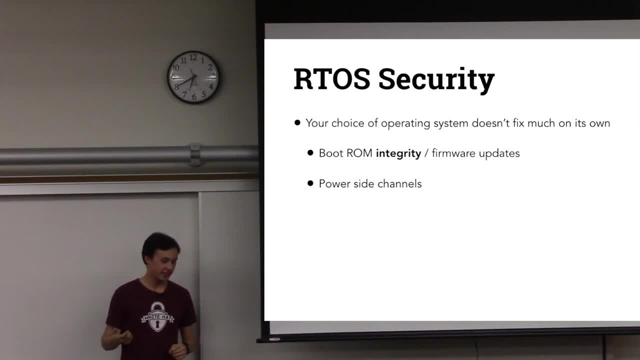 Your RTOS doesn't fix power side channels And all the foot guns typically found in C programming are still there Because RTOSs are embedded. You're usually writing C And you might think RTOSs fix timing attacks and they for some. 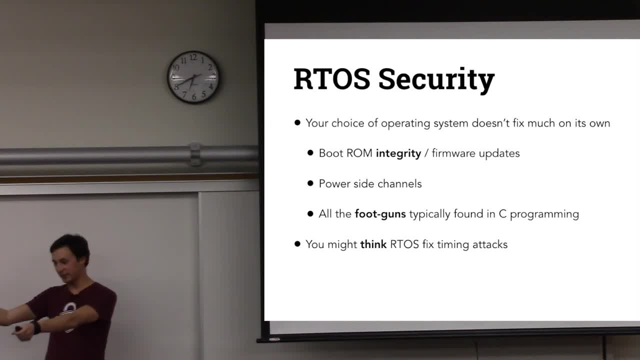 degree do And you just be like check password. It takes exactly one tick, But if it bleeds over into another tick then you're like: oh well, now they know it took a lot longer, Because it took a very discernible amount of longer time. 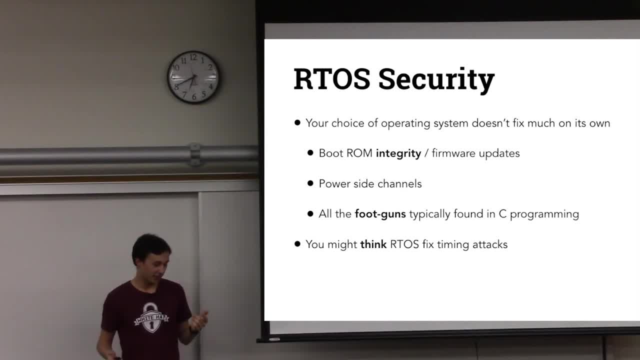 One good thing, though, is, since we're running on an embedded microcontroller, they're not typically vulnerable to speculation attacks. If you want to learn about speculation attacks, Nick is giving a talk about Meltdown and Spectre later this quarter. 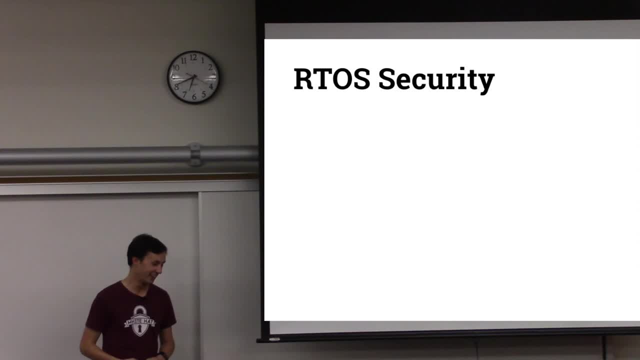 You predict you will, Yeah. So moving on with security, Free RTOS is the main open source RTOS everyone uses or builds off of. One problem with that, at least in terms of how they run the project, is the code is hosted. 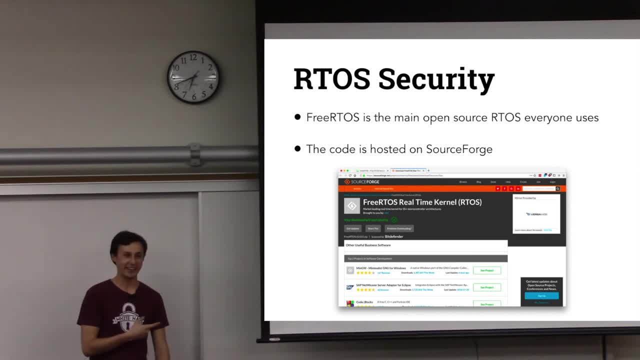 on SourceForge. So this is what it looks like when you download it. Like You get the ad, You get the other projects, You get whatever this is down here. Like this doesn't look like a safe download It, Hm. 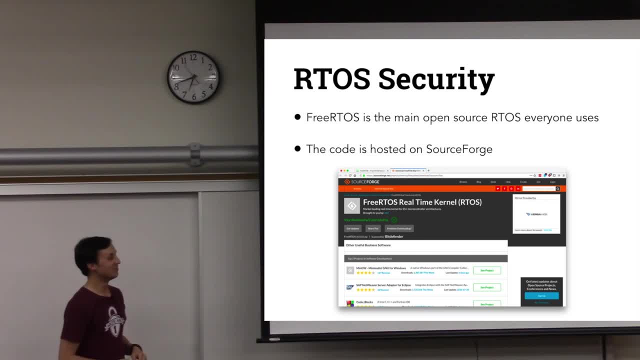 MalwareForge. Oh yeah, MalwareForge, Yeah. The thing is, though, like the operating system itself is small enough, you can just read the whole thing, And the other thing is there's not much functionality there and there's not much opportunity to. 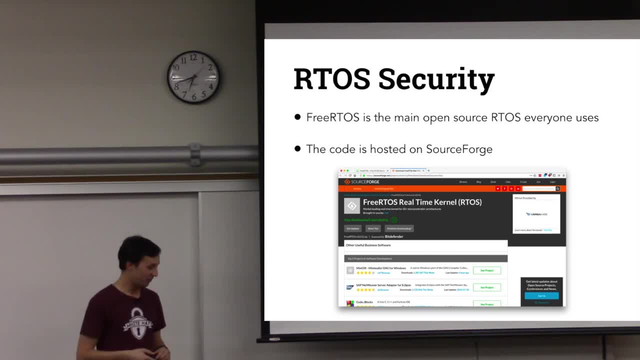 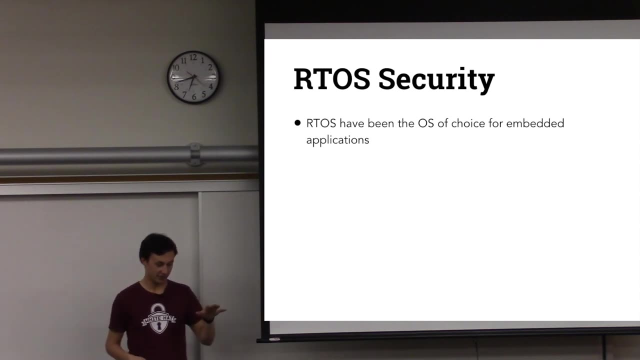 do much bad stuff in terms of just a scheduler, So You can be pretty sure that this isn't too bad. But the thing is, RTOS has been the OS of choice for embedded applications for a long time, And part of the problem there is networking stacks haven't been included in the box because 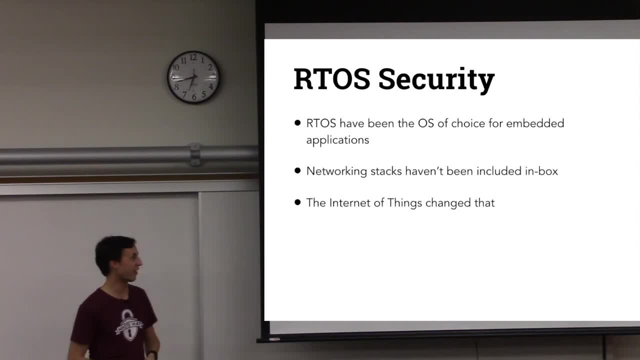 networking hasn't been a thing you did in an embedded application until the Internet of Things came along, And so the systems aren't necessarily built to partition RAM. So if you have a breach in any one task, it can just read the RAM out of another task. 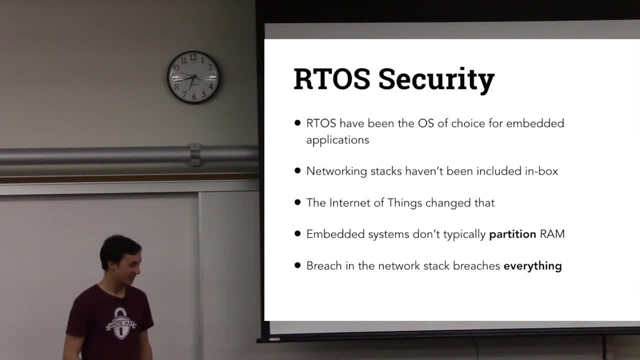 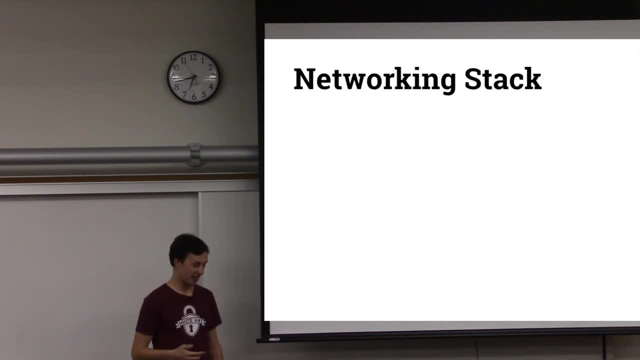 because the whole thing is just memory mapped. So if you have a networking stack, like RTOS's often have, just thrown into them, you have some issues you need to deal with because FreeRTOS doesn't come with one. Amazon actually renounced their own Amazon FreeRTOS. 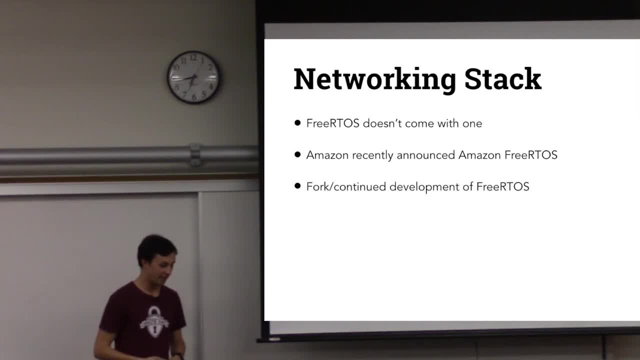 It's kind of like a fork or continued development of FreeRTOS, And the main thing it does is like We want a networking stack in this operating system, And then Amazon was like: hey, this one works with AWS, So The good thing about this, though, is it's hosted on GitHub. 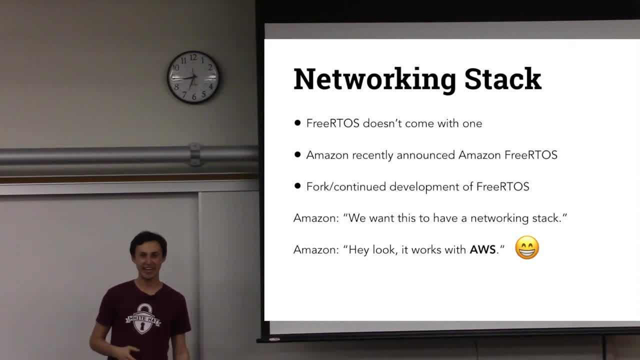 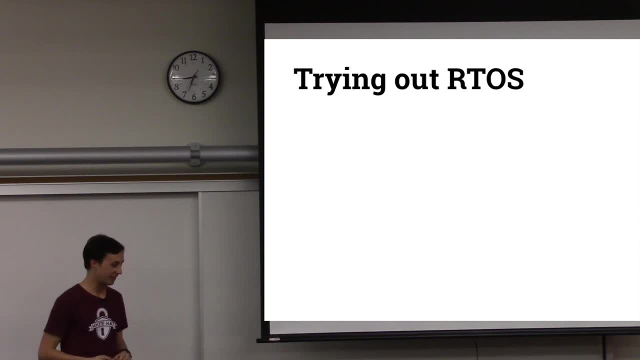 The other thing, It's also hosted on Amazon Web Services, So you can just be like: hey, Amazon, give me a copy. But- And I really recommend everyone, do try out programming a system with an RTOS, because it's actually really. 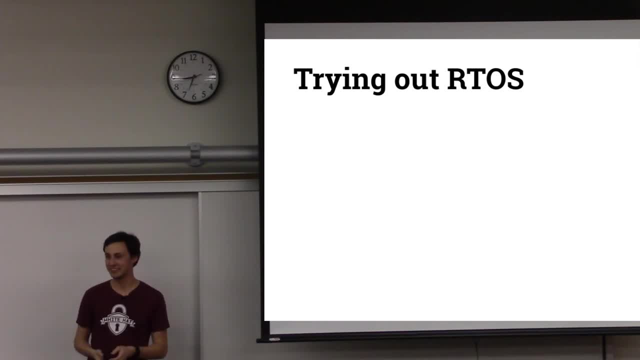 There's something really nice about building a system that just meets timer requirements, like that. It's like: oh, I want this thing to happen and this thing to happen, And then it does, And you're like, those are two different functions. 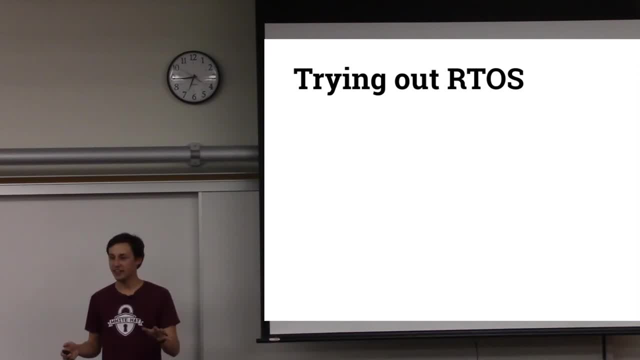 How are they running simultaneously? But so if you want to get into RTOS, you can take CPE 439, Intro to Real-Time Operating Systems. I took it last quarter with Professor Danowitz- Full disclosure. he's my advisor. Thank you, Danowitz. 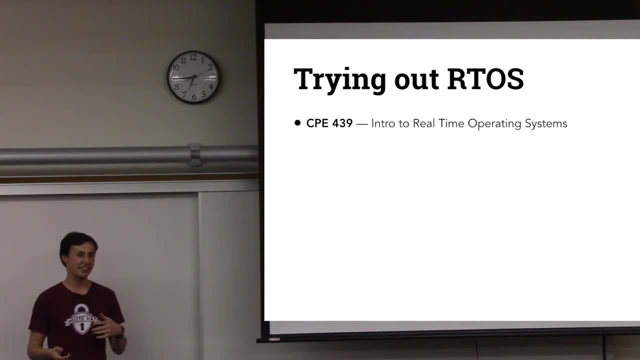 And the other thing is, If you don't want to do that, because it has some hard prereqs, like you really need to know VHDL in order to take that class in particular, you can just get a microcontroller and download it and run it. 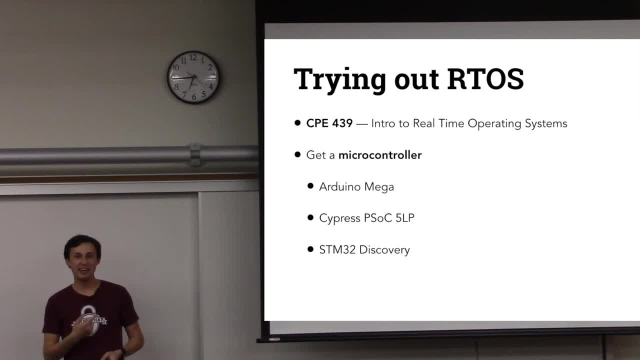 I recommend getting an Arduino Mega instead of an Arduino. I actually have a port of FreeRTOS for the Arduino, but it fills up the ROM with a couple hundred bytes left. So if you want to blink an LED at exactly the right time, it's your operating system. But no, Arduino Mega has enough space for it and enough things that you might want to actually like: have multiple UARTs running at the same time. Also, Cypress has some programmable systems on a chip which are ARM cores with some reconfigurable peripherals. I really like them. They have one for like 12 bucks, so it's a super good deal. Or if you want to do an STM chip, their discovery boards are pretty good And STM and NXP both have some chips that have like an ESP built onto them. 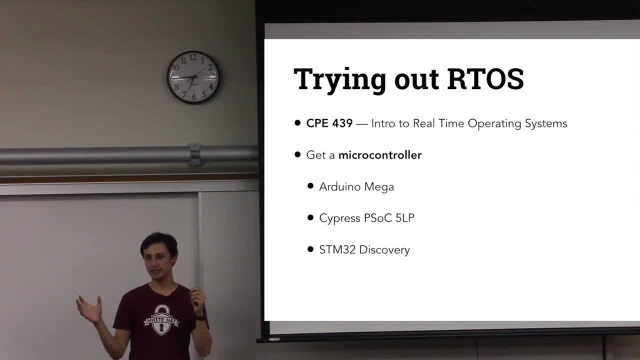 And then Amazon's FreeRTOS port is, like, configured specifically for those boards as well. Yes, Huh, What's an ESP? ESP, It's a Wi-Fi enabled chip, so you don't have to actually handle the Wi-Fi PHY. 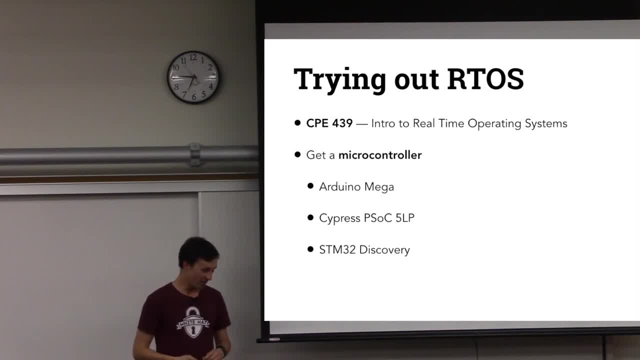 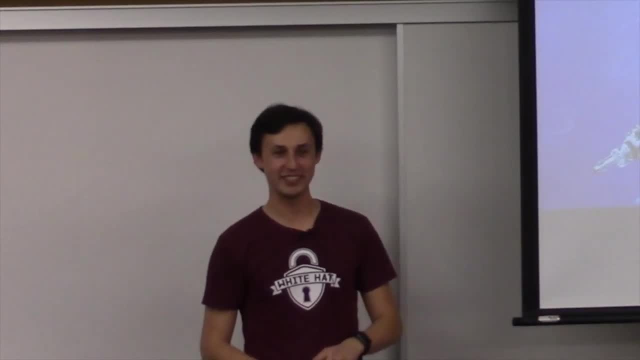 You just send it data and it sends it to Wi-Fi. So that's all I got. Anyone got questions? Aside from what, are all those acronyms used? I'm also happy to list off What is RTOS- RTOS. 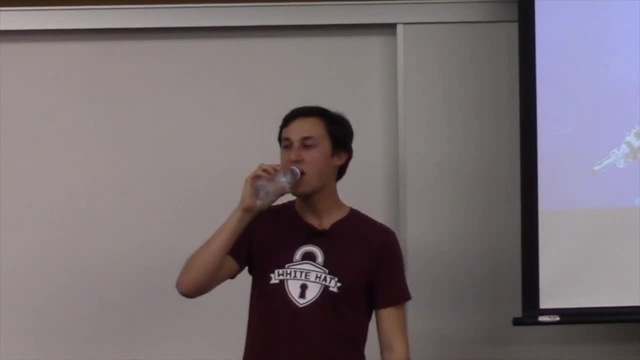 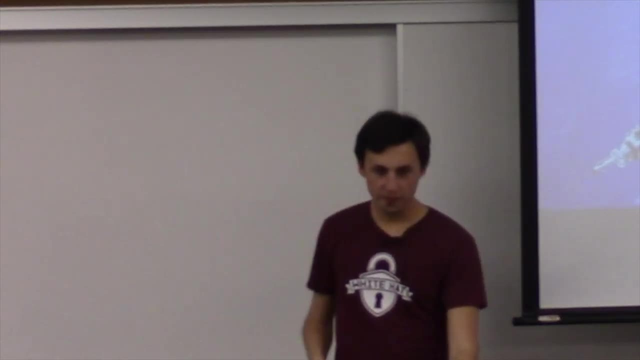 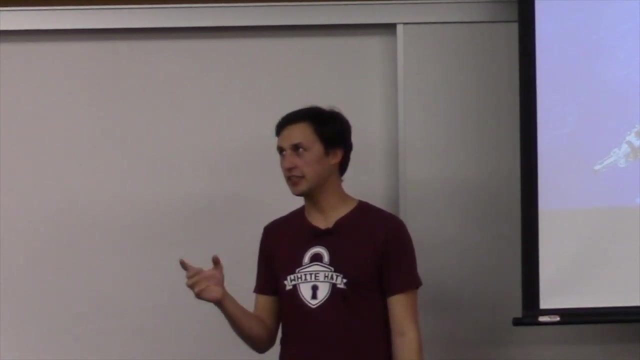 Real Time Operating Systems, So A? what does a chip do if it has nothing to do? What does it do if everything is blocked? When you write your system, you include with it an idle task, and so that's a special task that the operating system switches when nothing else is going on. 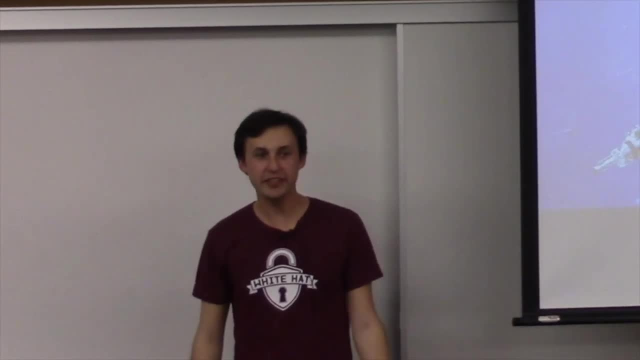 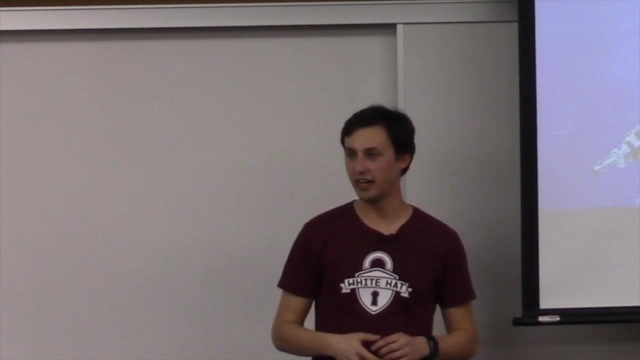 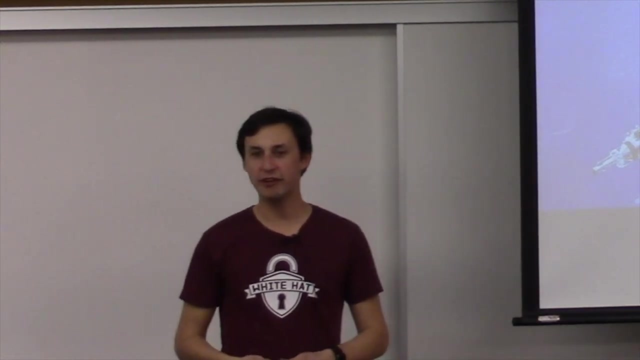 Typically it, By default, it does literally nothing. But you could also- be like during idle, i don't know- like clean up whatever memory i was using for, uh, dynamic allocation, or keep run statistics about how long i've been up or log stuff, or you can do whatever. 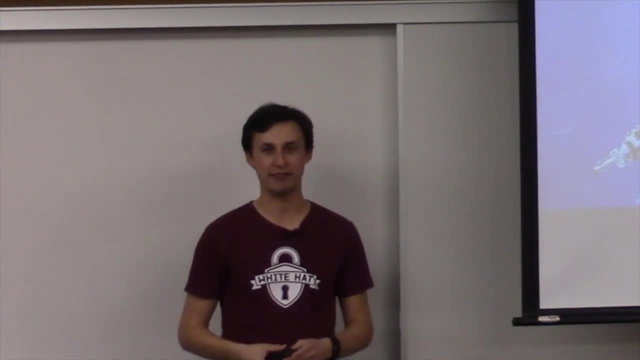 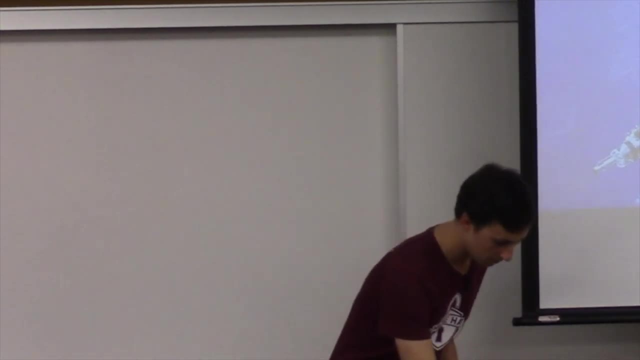 you want in an idle task, as long as you're willing for it to sometimes never run. so on the converse side of that, you said that often a microcontroller can have like more than one. i'm going to ask you a really specific question about how free our toss works. i 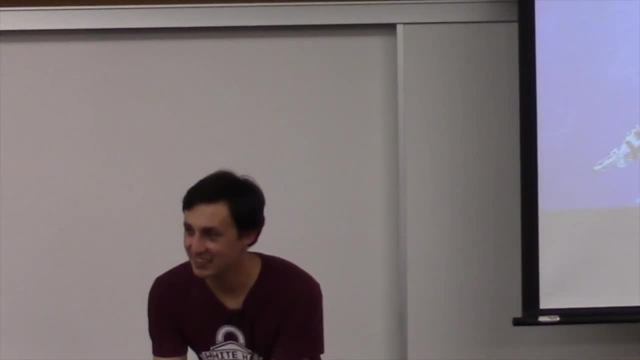 apologize, i mean i might know it so. um, so you said that microcontrollers often have more than one timer. is there a way to set like a super process like this: is the p, the p0 task that just straight up gets interrupted into when, uh, when it's not blocked? can you do that? i think? 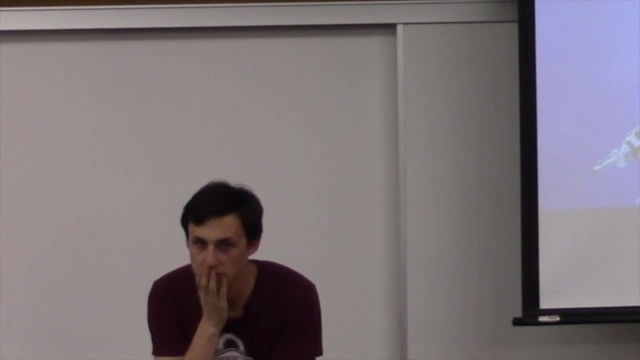 you just don't have anything if you set that up. if you want, you just put nothing else. if you want, like you can share variables, you can also just more abstract hierarchies and say like you want it to happen only on an interrupt, i want it to. 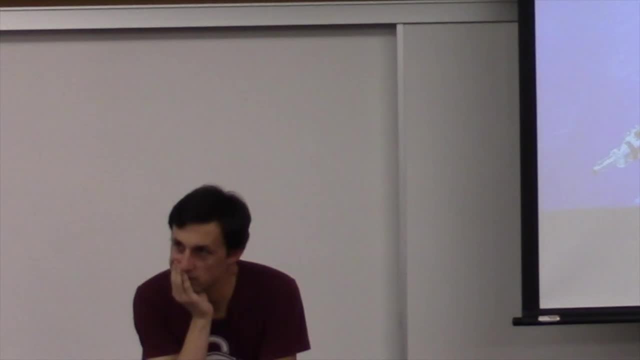 not even need the r toss. i want to have it on the side so it doesn't even. so it starts running even without the test too. yeah, um, yeah, you can do that. like will free our toss be like wait, no, i was using that. or you probably need to like tell freer toss that something happened. 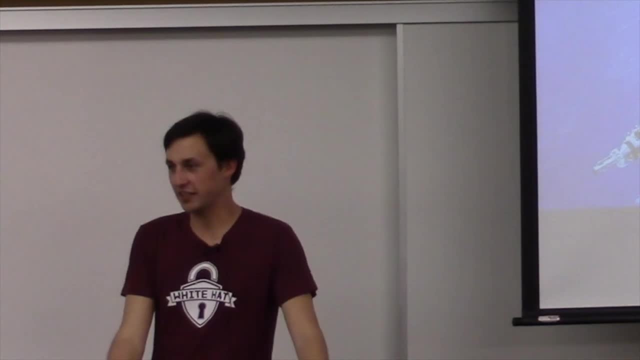 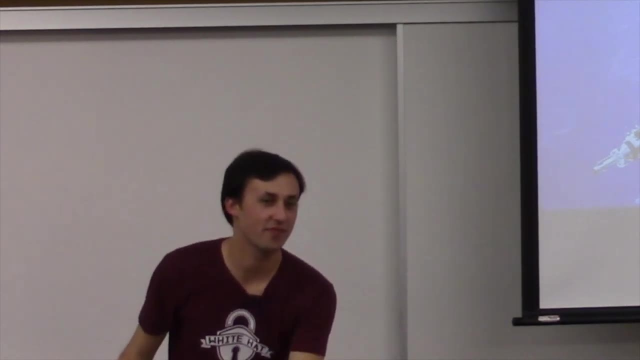 um, but no, i mean you can set up your interrupt service registers to do all the anything you want. cool, i have another follow-up question. yeah, how do you use it? um, i mean by default, it's like maybe a couple milliseconds to a couple hundred milliseconds um. 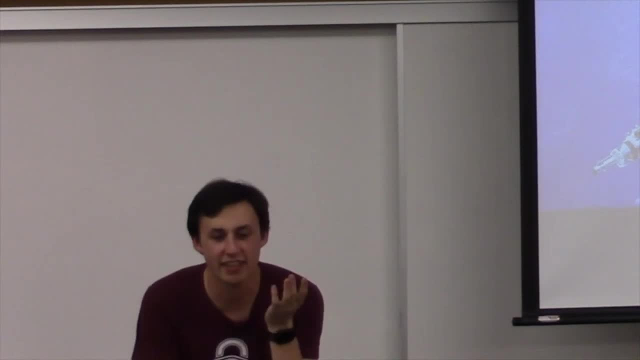 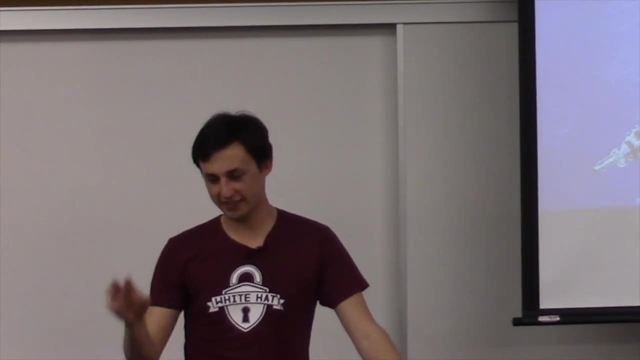 i mean like a couple milliseconds, like maybe a millisecond here, a millisecond there it's. it's however long you want. in fact, when you run free r toss, you just go into the configuration file and you're like: i want this number of uh ticks, this, this amount of time to go by for tick. um, basically, you just calculate, you just. 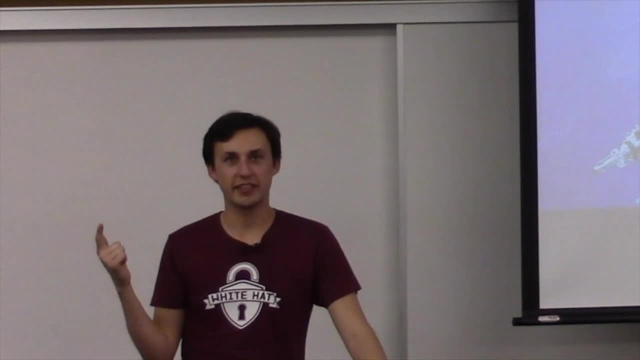 you just give it the system, clock speed, the timer configuration and the number of milliseconds you want to run between ticks and it calculates, uh, everything it needs to run the ticks at that length. you get a follow-up, all right. uh, you first. um, so the task finishes before the check is up, because 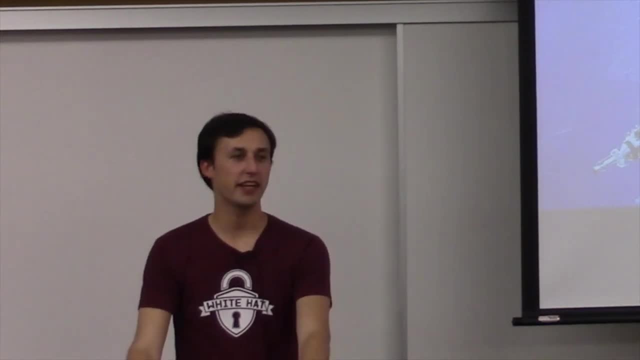 it's just like: wait, yeah, so if a task blocks, it'll just wait out the rest of the tick. um, uh, you could probably hand back control to the idle task if you wanted to, but ticks are usually short enough that it doesn't matter. uh, the multi-questions. when does our gos have a graphic user interface or as a command line? 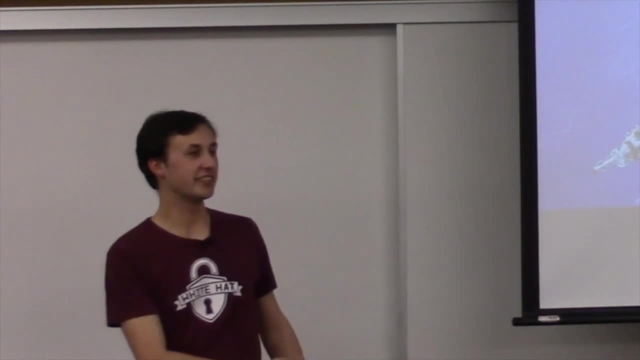 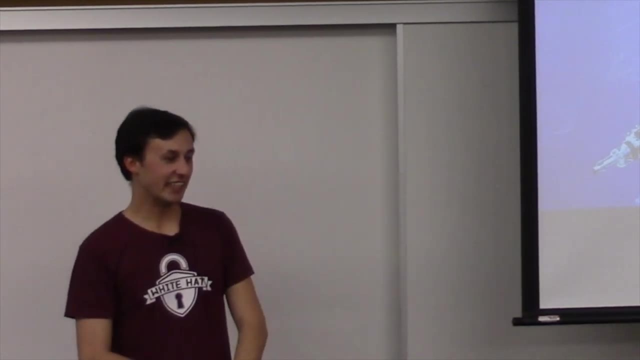 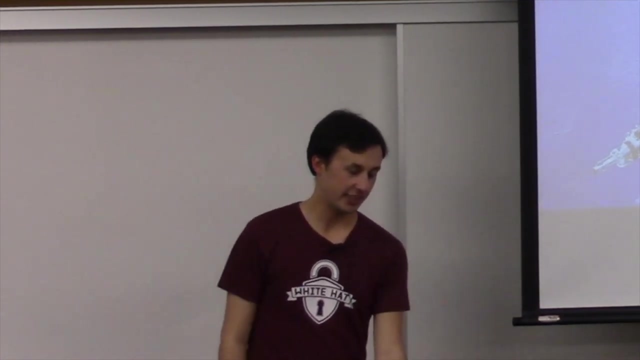 um, well, so it's not an opera, it's not an operating system like you're used to it's. it's for like. like they don't typically have screens attached to them or keyboards. like you have general purpose input and output that sends one ones and zeros to devices you might have like a serial port. that's like physically just. 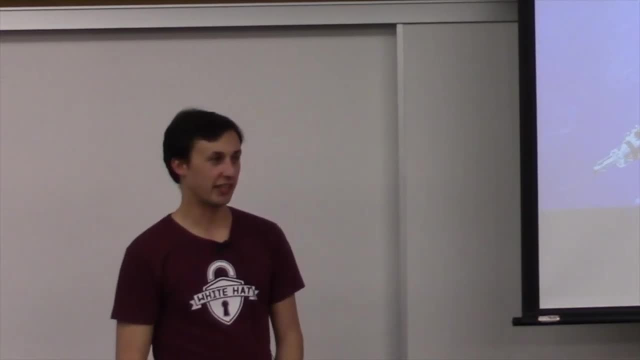 like serial pins, um, or just an i squared s bus or i squared c that sends data to another chip on the board. okay, and then would anything start to go seriously wrong if you said it's like a really long, like uh, interrupt time like one second or something. i mean, the only thing that would go wrong is you might miss your time requirement. so the finer the tick is, the more often you get interrupted, but the more likely. but the smaller window you have before a higher priority task that's become unblocked starts running. so if you have a tick length of 100 milliseconds and you want something to run, every thousand milliseconds. you could be a thousand plus or minus a hundred if you have that, but if you have a 10 millisecond tick length, then you're a thousand plus or minus 10 milliseconds. yeah, the smaller the tick is, the more time you spend in the scheduler. 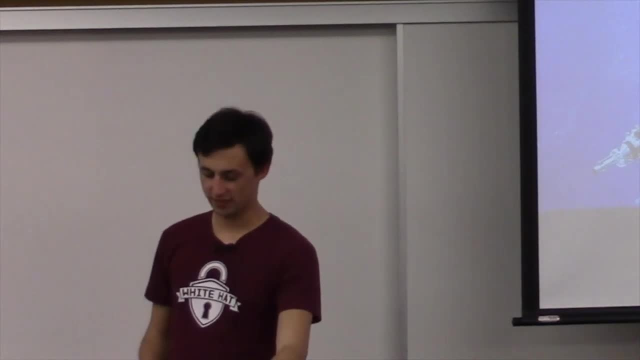 okay, so this has nothing to do with my original line of questioning, since it's a whole new one. uh, you know, i have to finish the original line. please do that. i forgot, okay, um, so let's say that i i've got my. i went out and i bought my shiny new, my shiny microcontroller and i want. 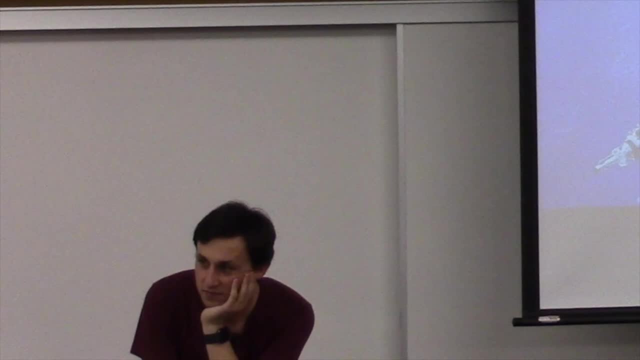 to put some some free r toss on it. what would you recommend as a good beginner r toss project? um, what's the coolest thing you could build with r toss? and, like any protocols or whatever you've done, we can only do it for a second. see, that's what i don't want to do. i mean anything. 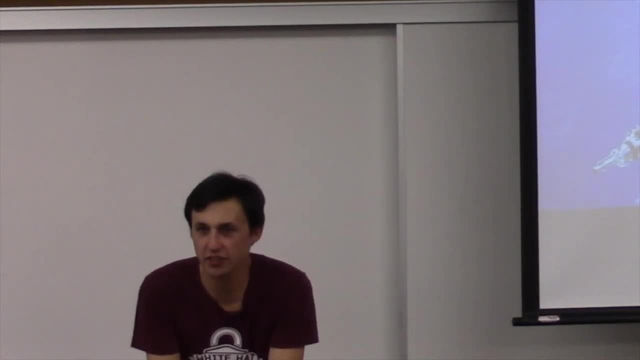 you might want to do on your computer. just offload that, to like offload two different things onto this microcontroller, just send it over the usb serial and be like: i want to write this program, but i want it to happen on this computer instead of this one, and then, since you're doing two things, you can.